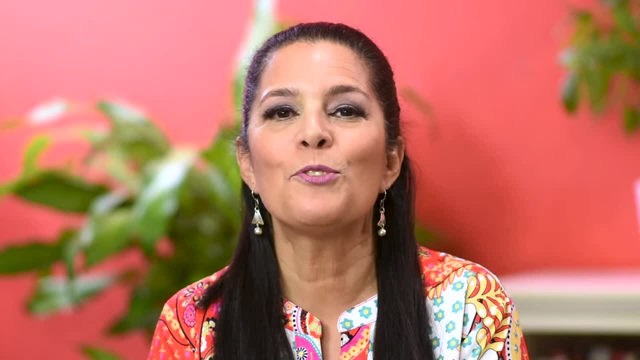 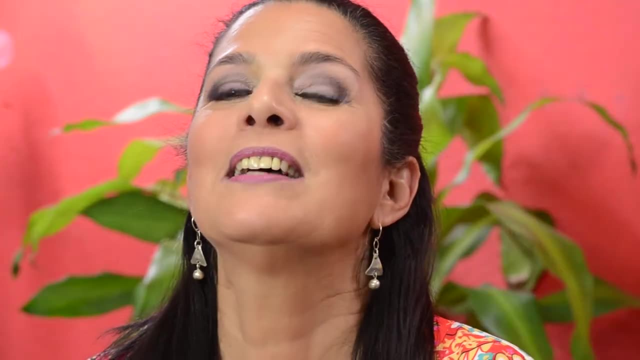 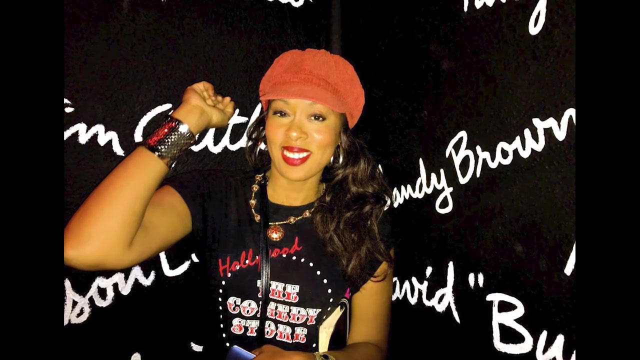 Hey, Common Censor, If you're looking for acting tips, industry insights, interviews or life lessons, you have come to the right place. Today I am just Elated to get to introduce to you one of my dearest, bestest friends in the whole wide world. 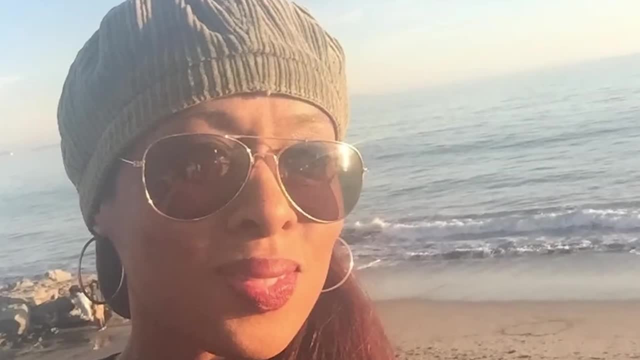 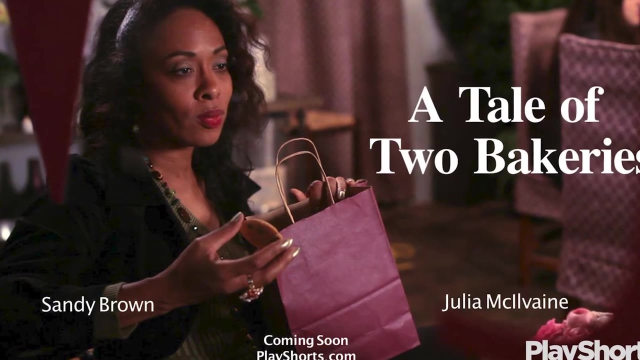 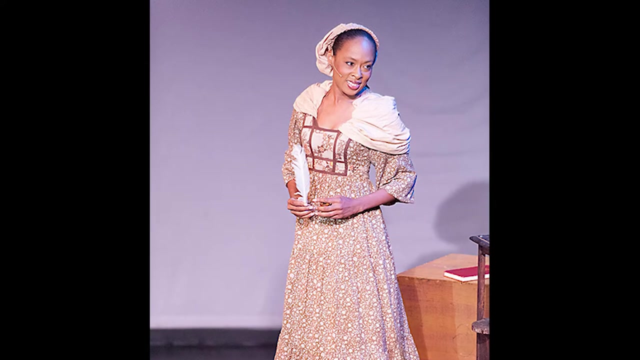 She is an award-winning actress, a comedian, a writer, producer, solo performer, singer and sketch performer who unleashes entertainment that tickles the mind. She is one of the funniest people I know and has been referred to many times as the Black Carol Burnett. 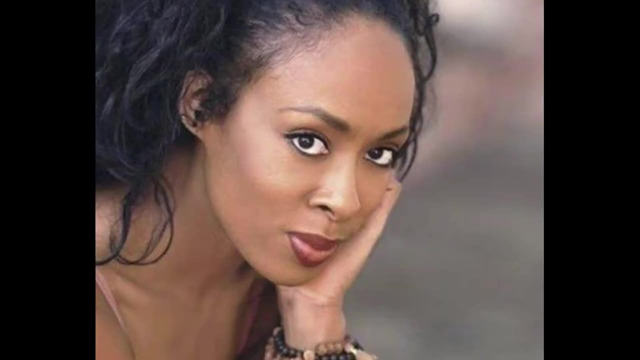 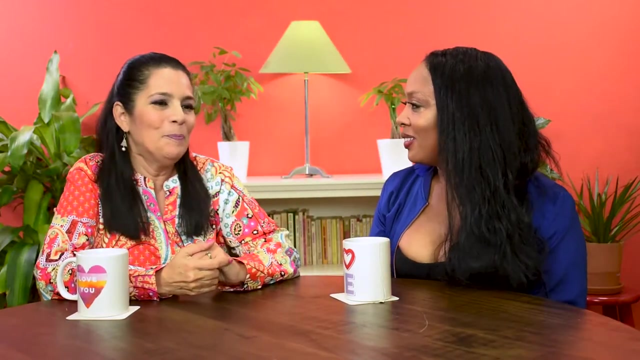 Please help me. Please help me welcome Miss Sandy Brown. Yay, I thought, Sandy Brown, Hello, I'm at the table. You're at the table. I'm at the table, That's right, You're at the table, girl. 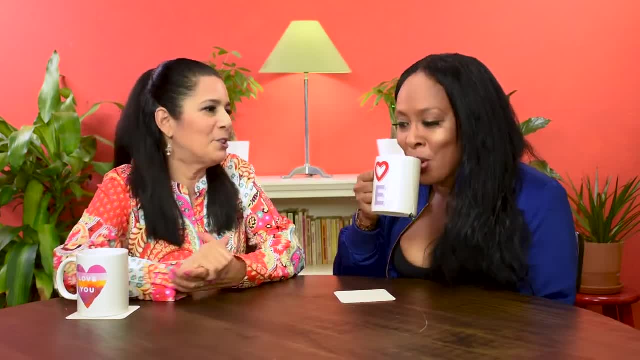 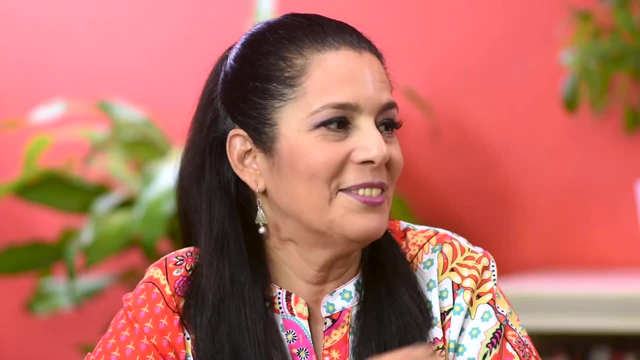 I like it. I like it. So I want to talk to you about your one-person show. Oh Yes, She Did. Oh Yes, She Did. Now give me the whole title: Oh Yes, She Did. Oh, that's it. 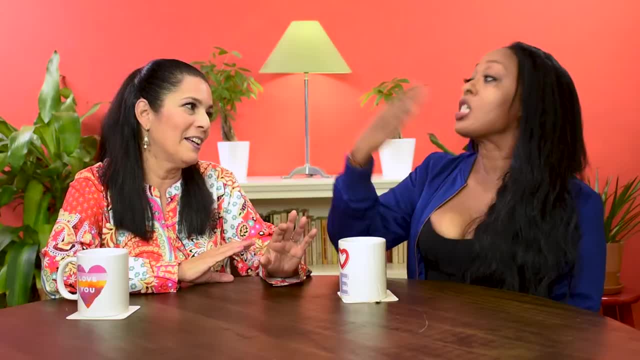 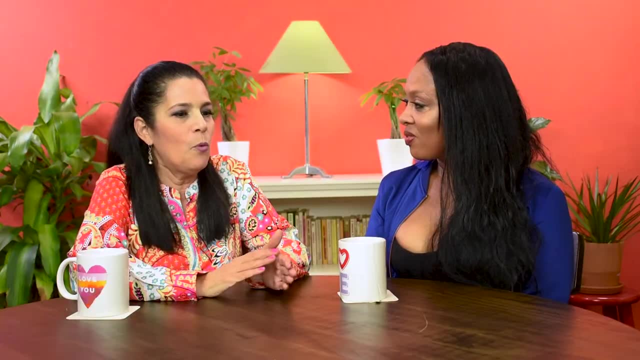 Oh, the main title is: Oh Yes, She Did Slaveship to Spaceship actually. Oh, okay, From Slaveship to Spaceship. Yes, All right, Very good. Now what inspired you to come up with this piece? 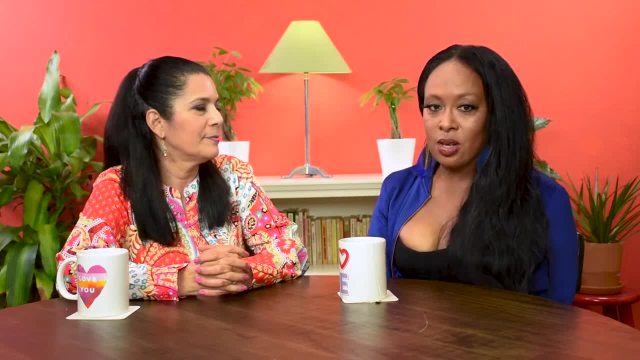 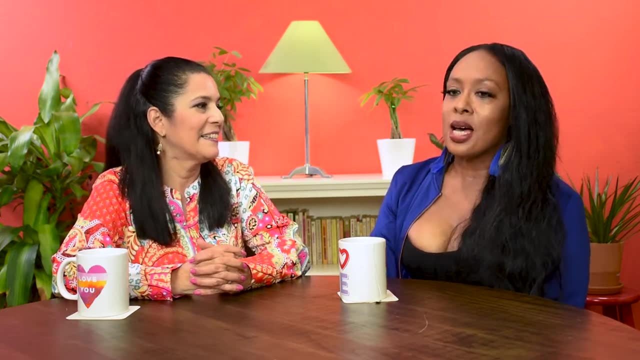 I had a different one-person show originally and it was a futuristic show regarding the apocalypse and everything that's going on in the world, And I was asked to present a show for Black History Month And I said, okay, I'll pull that together. 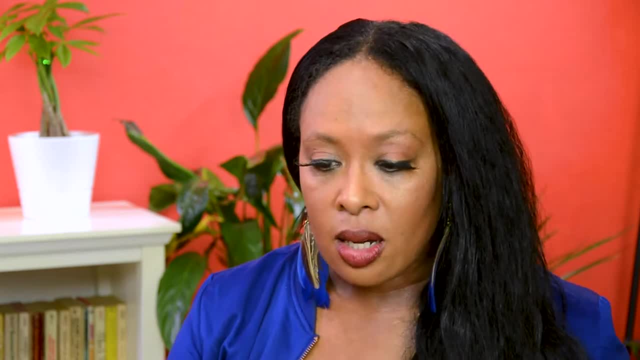 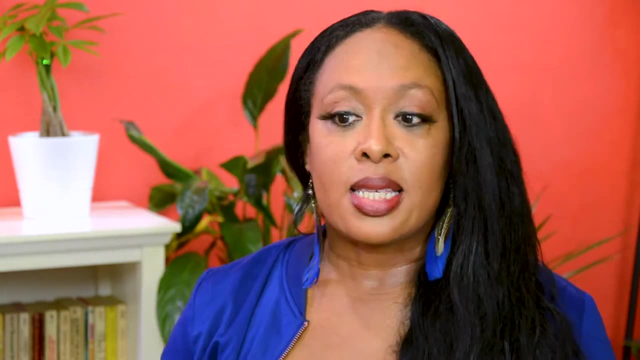 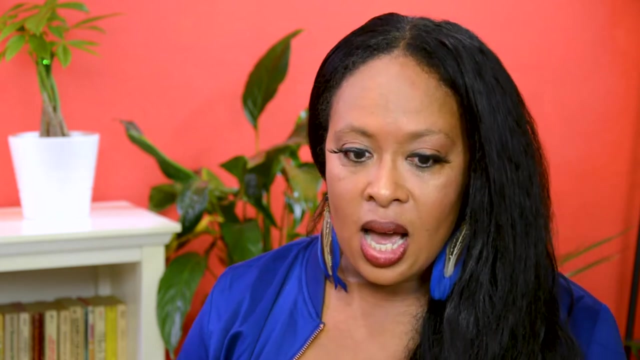 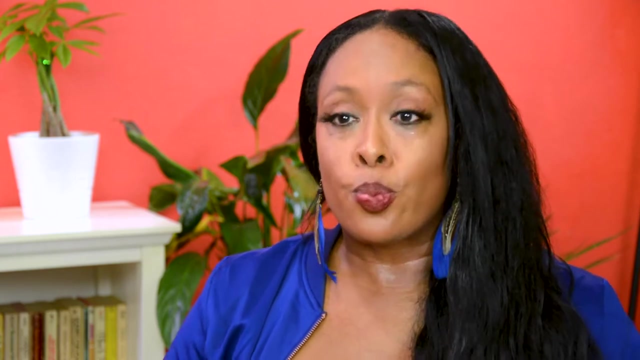 And after studying one-person shows with Adila Barnes as well as a few others, I said: this is a great thing that we've learned to do for Black History Month, When I went to study for each of them and I did the show. I did it the first time and it was so overwhelming because for me it wasn't just to put on the outfit and speak about the person. 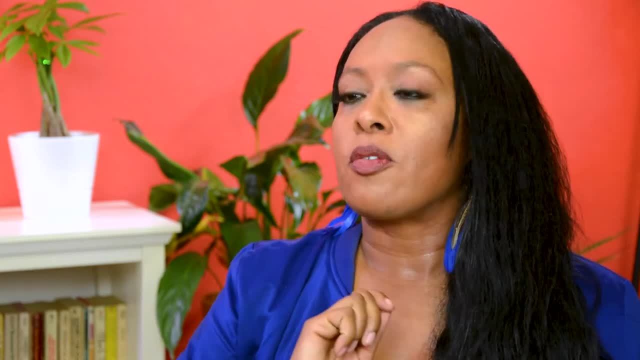 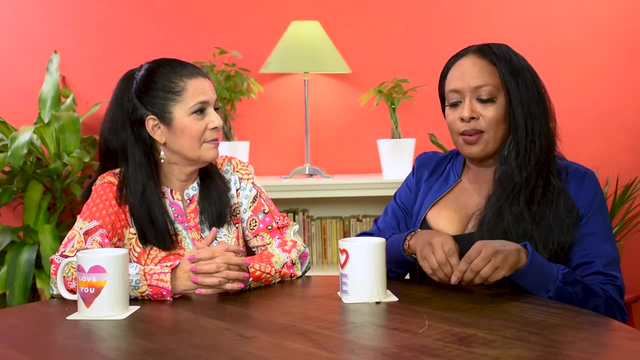 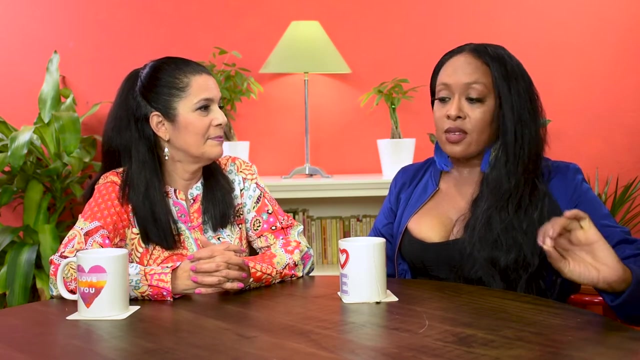 It was to embody that specificity, It was to embody that specific, pivotal moment in their life that made a change, the sociological change that they made. And so to understand that- and my show spans 400 years of history, so I have literally from Slaveship to Spaceship- 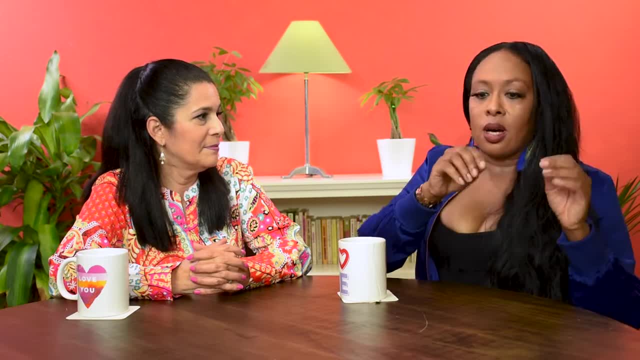 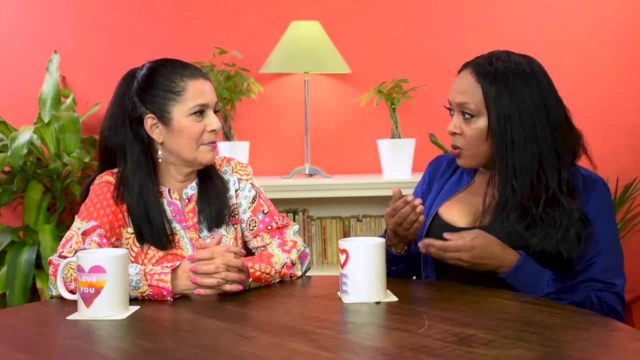 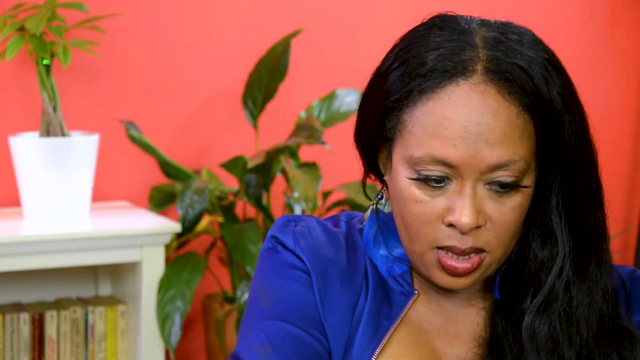 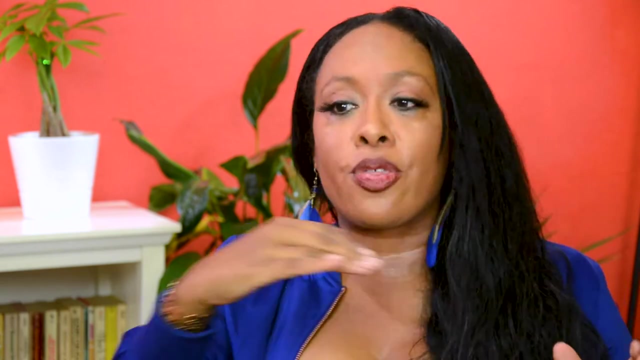 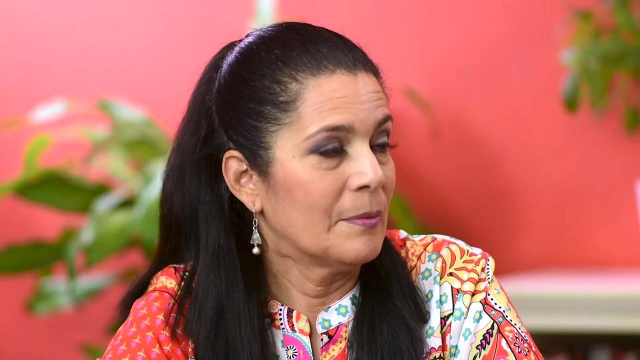 And so each person embodies a specific time and space, And so you can't just play them all and expect there not to be layers. They overlap on one another And one stands on the shoulders of each, So I needed to learn all about this time and period, the pre-slavery as well as slavery. you know the 1600s all the way through to modern times, because you can't understand one period in history without understanding what fed into it and what happened afterward. 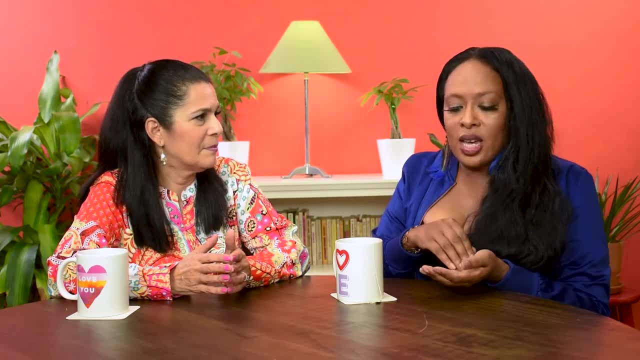 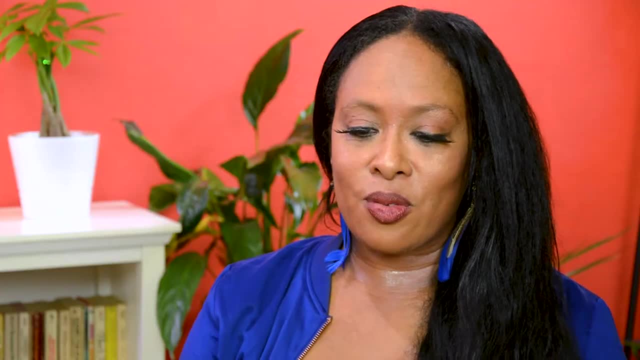 I mean, it informs all of that. So the more that I, you can't just throw that together. And I learned that when I did the first one- And it was so odd because the physical, The physicality of it, and the costumes, because I wanted to literally give you the full dressings of each. 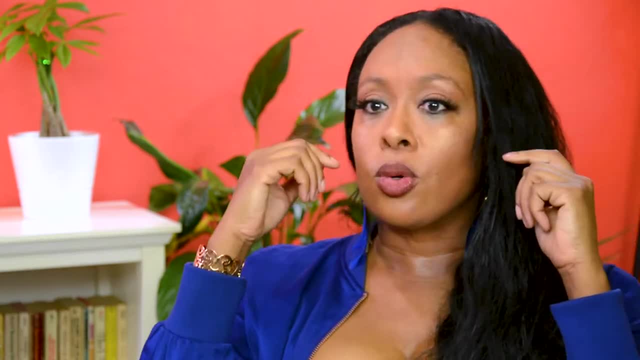 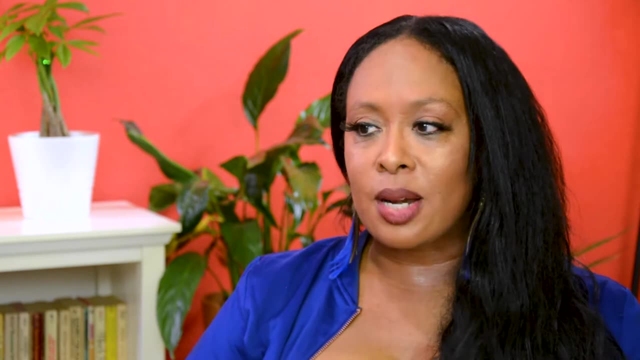 Because some people do the solo show historical and will do an idea of the character- a scarf or a hat- for easy change. That's fine, But to me I feel like you learn a lot about somebody by their clothing. We know a lot about each other now from you. know the different clothing styles. 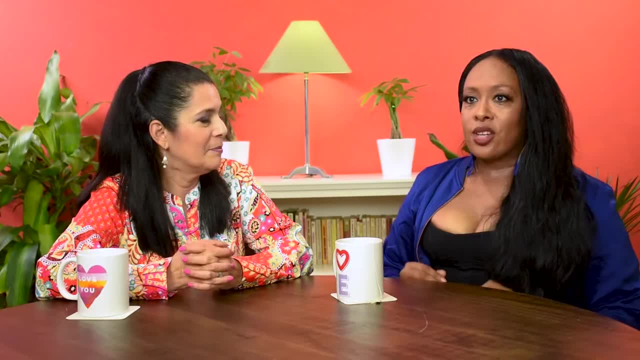 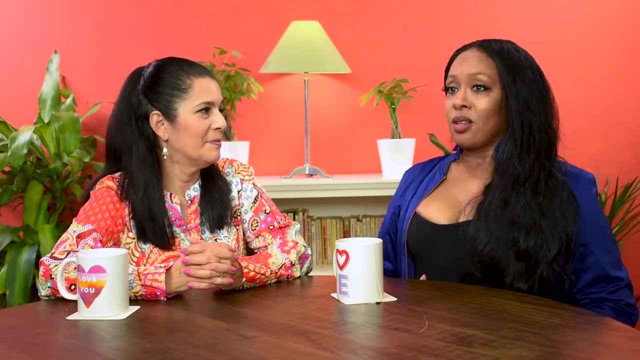 Now you can clock something and understand why something is so, And so you carry yourself. I think I mentioned this before to you. You carry yourself, You look different, whether you're wearing a corset or the chic. you know what I mean. 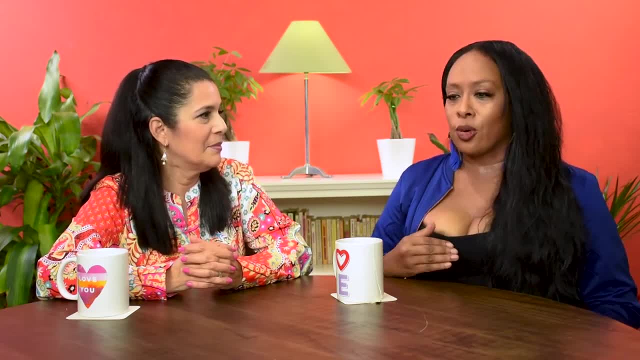 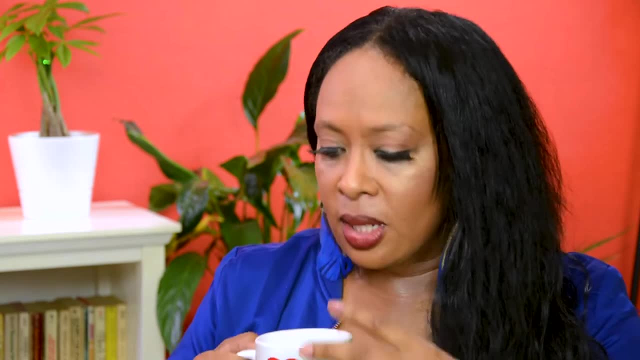 And so that informs about the time, too, and what the people are going through, And so it was very important to me that it was full dress, and the hand props and everything like that were were important to me as well, And so I did an initial performance of it. 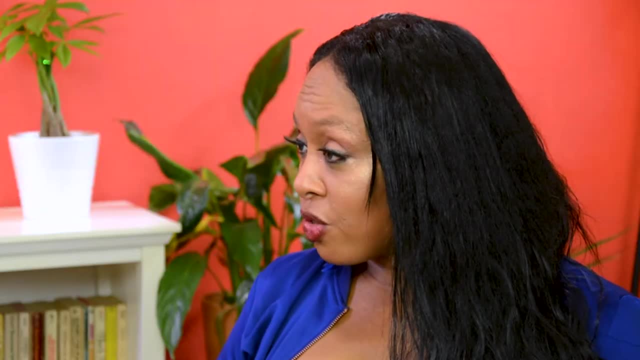 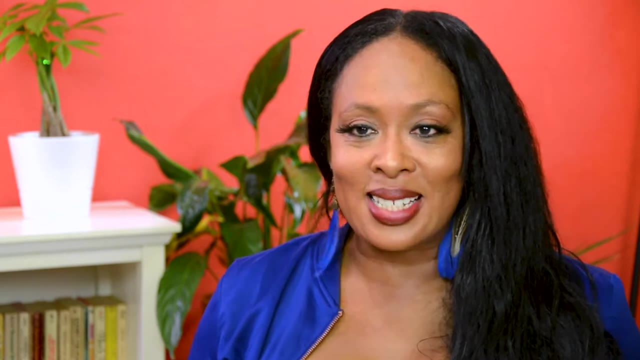 And what was interesting is that I wasn't familiar with the idea of having to change clothes for each of them, So I hadn't adapted the quick change method in terms of Velcro, And you know. so I'm literally in there doing the full dressing. 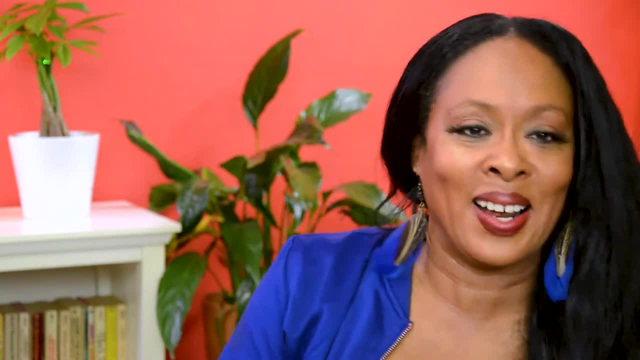 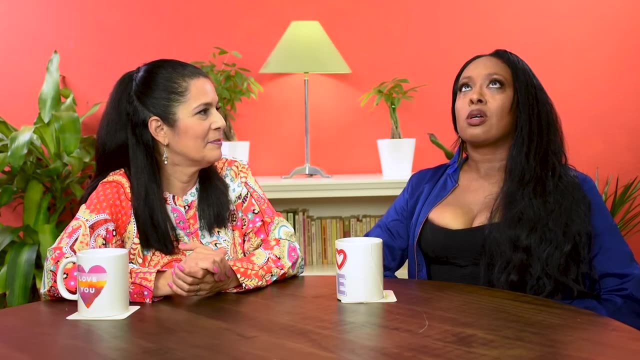 And I'm sure the audience was like where did Sandy Brown left it? And then I finally, you know, when I got home the night after the show and they left the show and it was, it was, it was so fulfilling to do it. 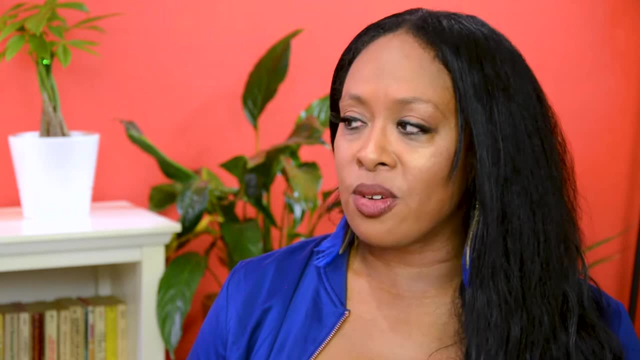 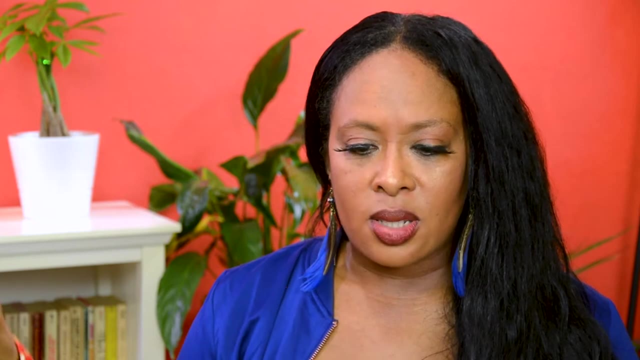 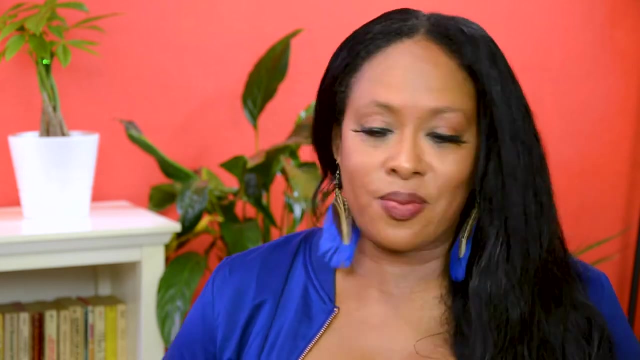 When I got home, I slept for 24 hours- The energy of it And also- but I also knew the outpouring, The outpouring, The outpouring of energy to, to, to, to create it, And also, when I got back and it just, and it was just literally, for lack of a better word, whoever received this or not- there was a spirit that said: rest my child. You know what I mean. And it hit over me And I literally looked at the clock and it was 24 hours later. I've never slept that long in my life And after I did the show I said: to continue to do this, I have to go deeper. 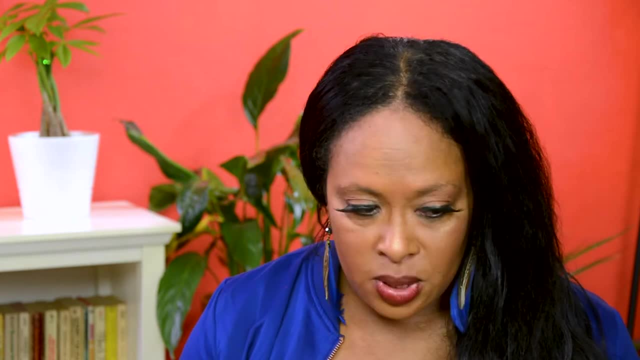 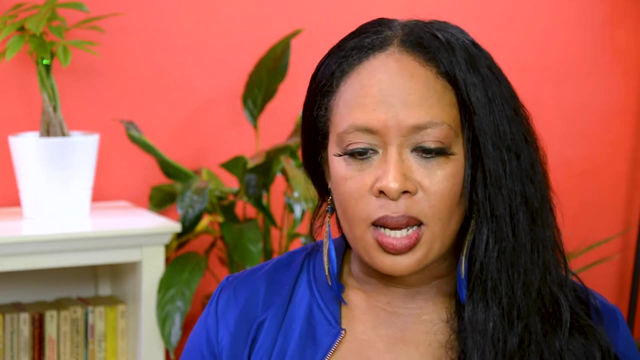 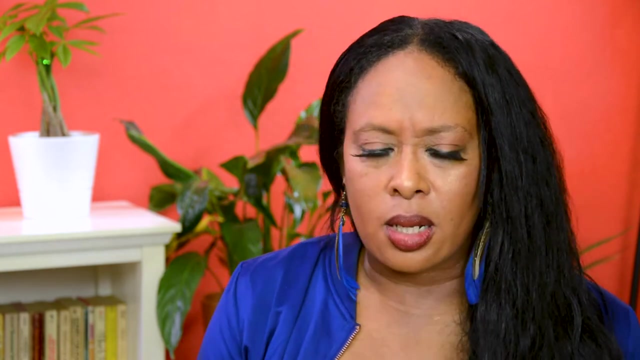 And I went deep into the woodshed And deep, deep, deep, deep woodshed study of each and every one of them and the histories surrounding them. That's why it's such detailed with with the costumes and things like that, because it informs that they're, they're, they're way in the world. 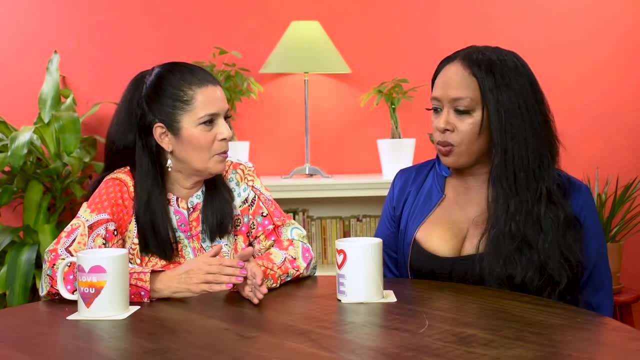 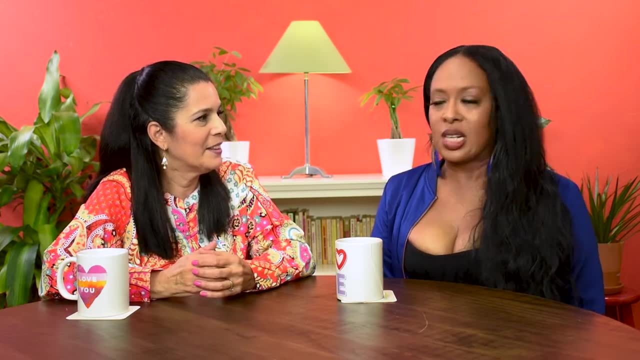 And I started doing. I started, I started doing it when I when I did it full out the first time- And it was my sister who helped me name it- because I said: oh yes, she did it. Oh yes, yes, she did. 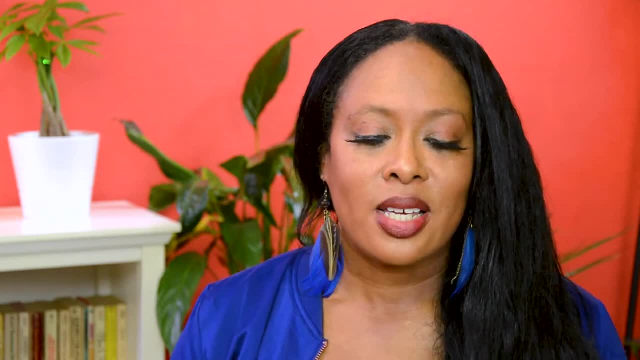 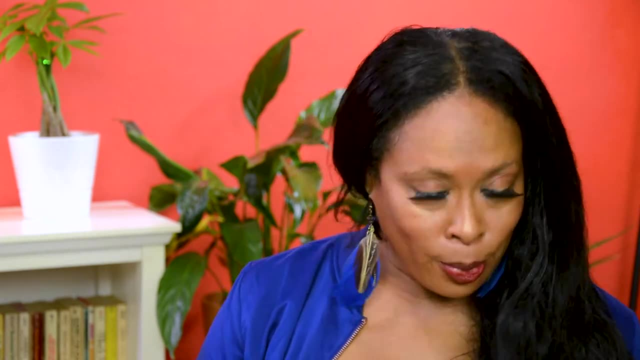 You know, you know she was like no, no, keep it tight. She and a crew of people helped me do it for the first time at the Barbara Morrison Theater in Los Angeles, in Leimert Park, And this was after you did it the first time. I did it after I did it for a college college. 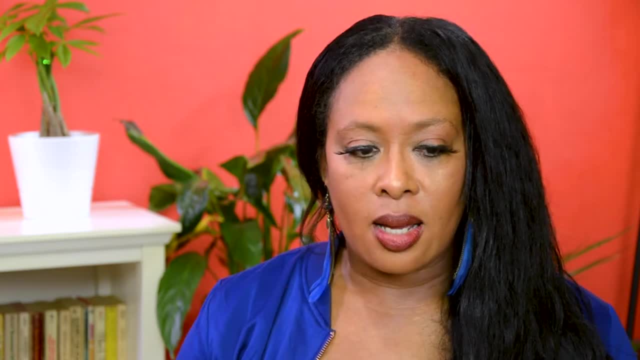 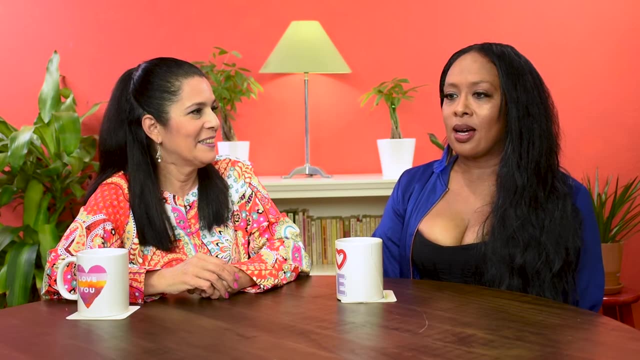 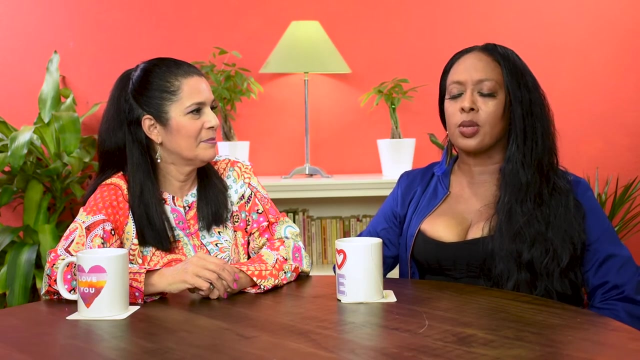 And then when I did it from there, there were more people on crew. Then Were in the audience and and I was, it was, it was, it was an exhausting turn And I said, do I want to do this? And it spoke to me again. 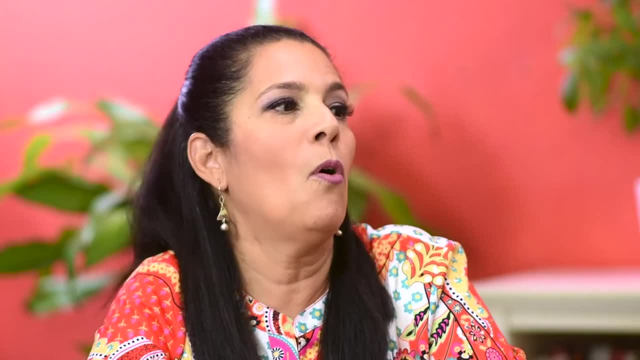 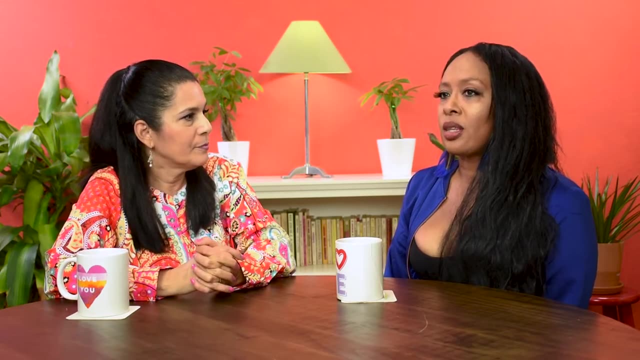 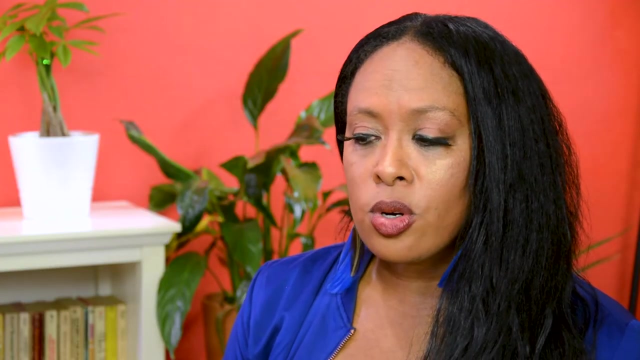 No, no, You do want to do this. What made you want to go all the way? Because that's you're. you're covering 400 years. I'm covering 400 years And and some of the women are so well known that that they bring out every year in an honor in celebration of Black History Month. and others weren't so well known. 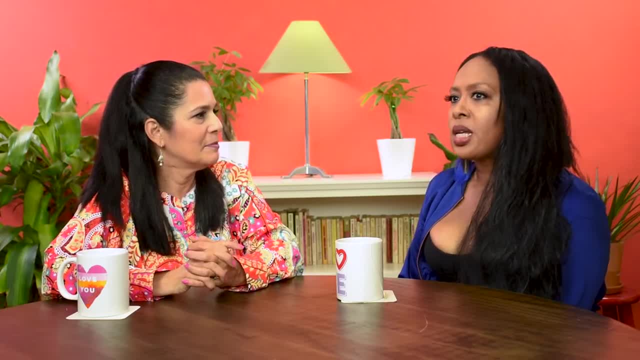 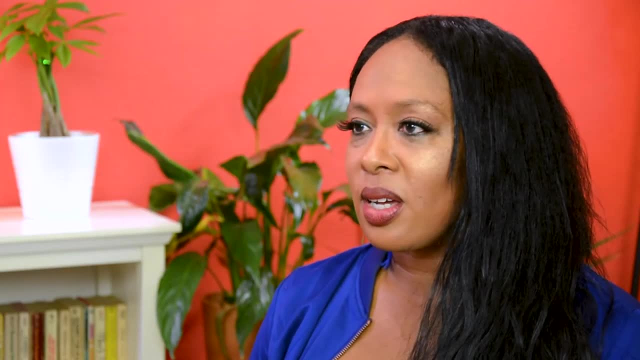 And And I had felt that I had done a level of study in my life and and education. No, these people and I, I was affected by the fact that I didn't And I said, well then, I just stepped into that. 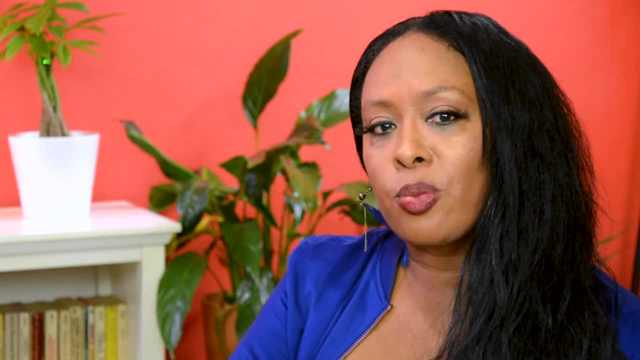 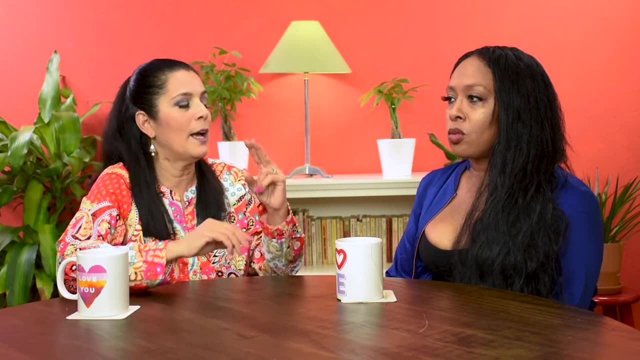 Well, what I stepped into that void and said: well then, I will present those so that other people know And, in fact, on. So let's talk about who's on it, because you actually have two shows that you broke Broken up of these women. 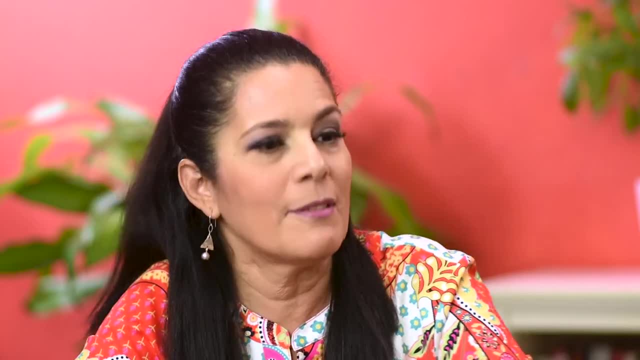 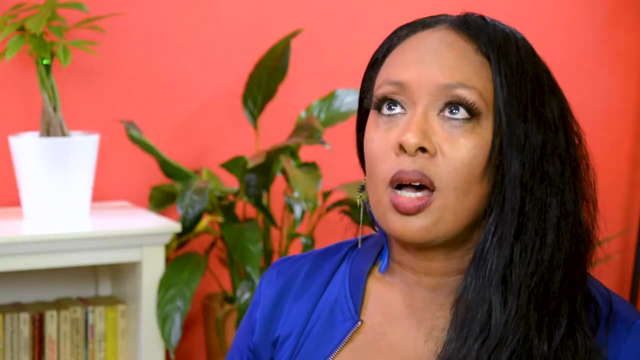 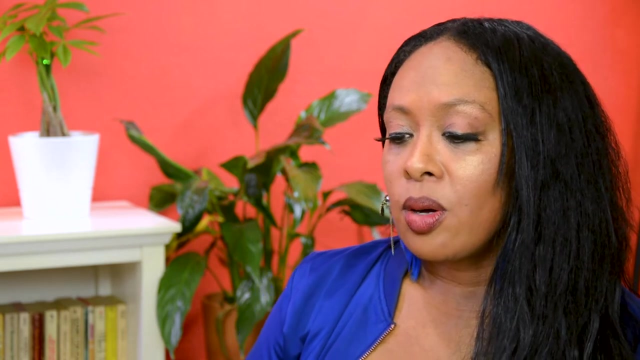 But on the first show, who are the, the stars of the first show? Yes, we have Phyllis Wheatley, We have Harriet Tubman, We have Madam CJ Walker, We have Josephine Baker, We have Billie Holiday. 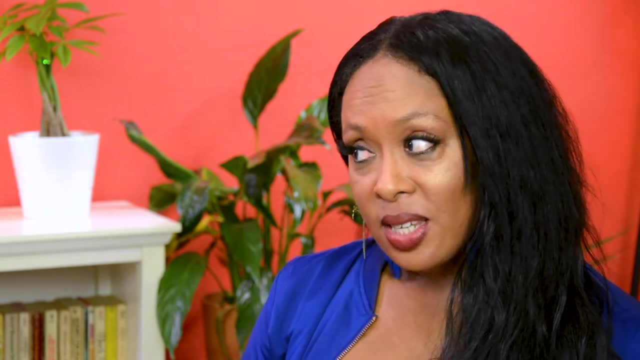 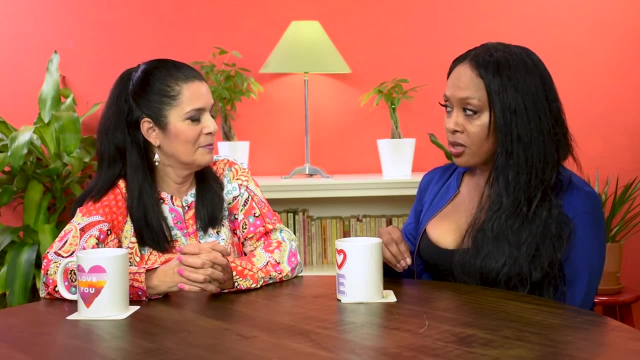 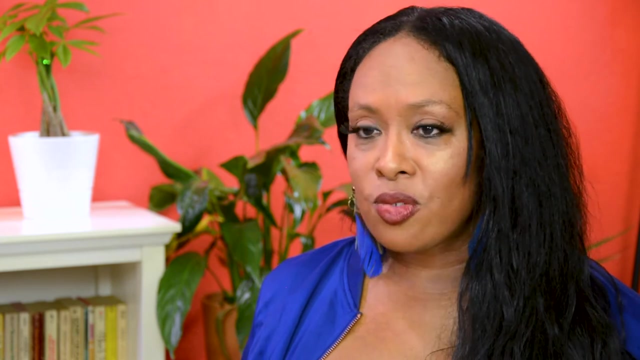 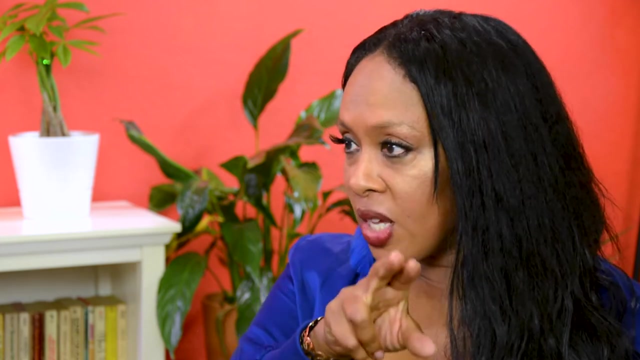 We have Rosa Parks, We have Angela Davis and we have Shirley Chisholm. Now, what's interesting Is I did all the the, the graphics and ideas for it, and the idea of it was to have the iconic banana skirt of Josephine Baker as international spy and performer, in the center along with all of the other women. 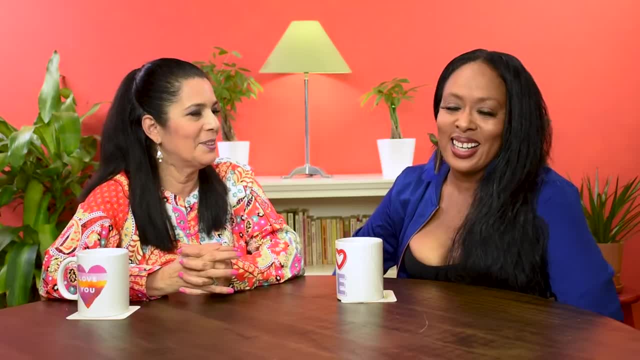 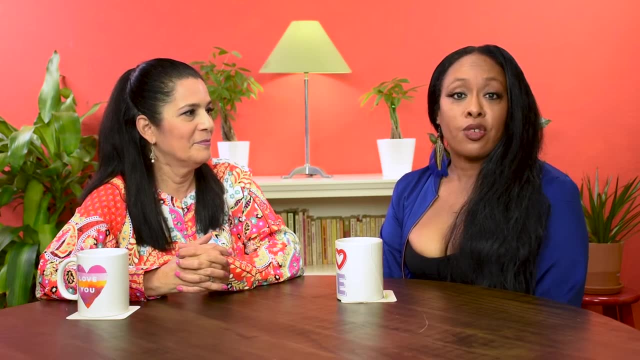 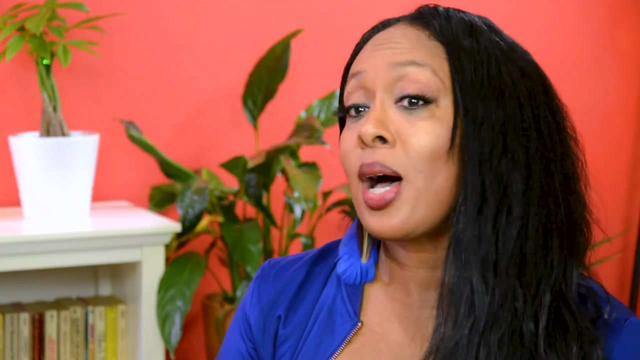 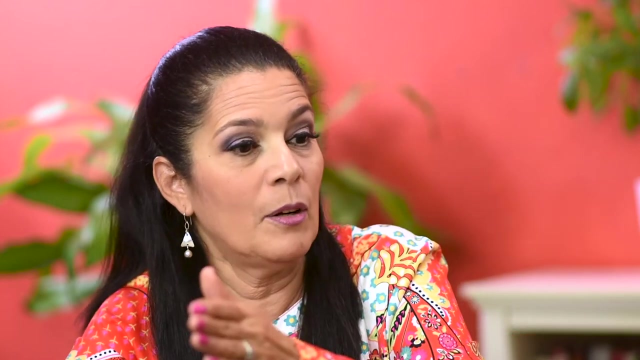 So tell us who Josephine Baker is. Josephine Baker was a entertainer, film star, actress, dancer from vaudeville days On up to the talkies, And she was also a spy. And she was she. she also left the country, left America, left America and and became a citizen of of France. 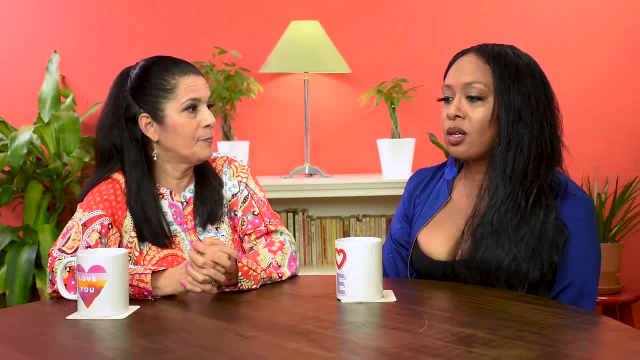 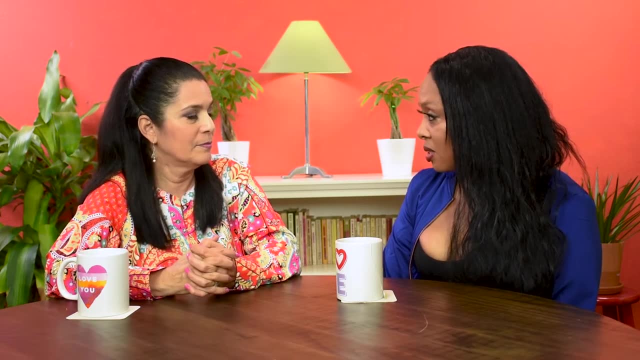 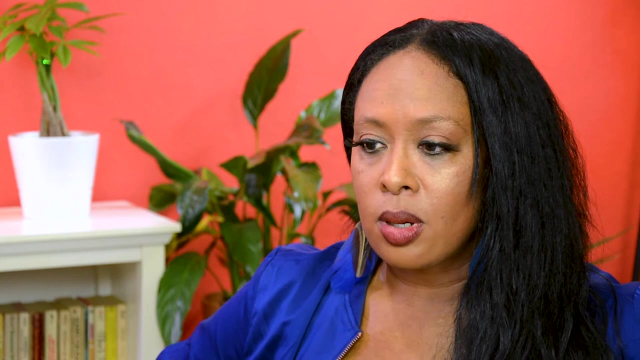 Yes, yes, There was. there were a lot of issues for black Americans at the time and a lot of performers had the option to go overseas And she said: I will do that. I will definitely do that, And what happened is the evolution of her life. 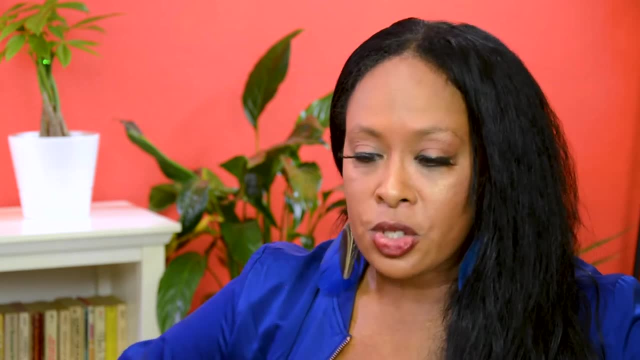 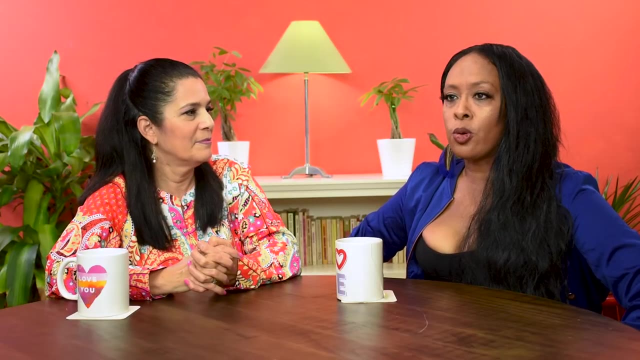 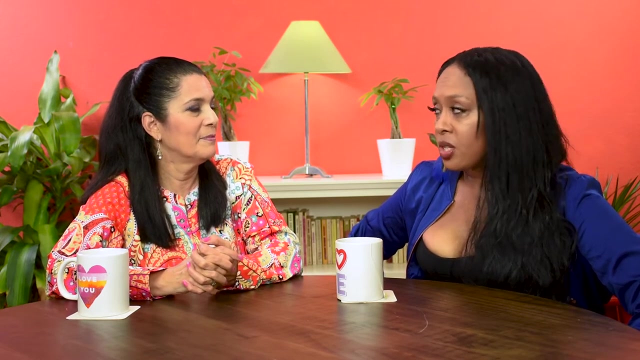 She was. she was confronted by Goebbels and it was part of the Nazi Party and people would write about her and she was bold and she would. she was outspoken and she would speak up about it And she would also hide, hide people for safety in her home. 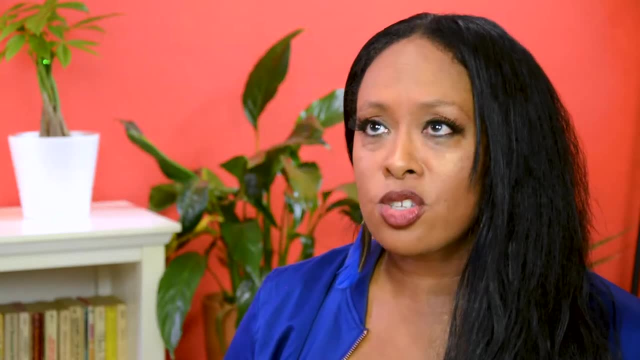 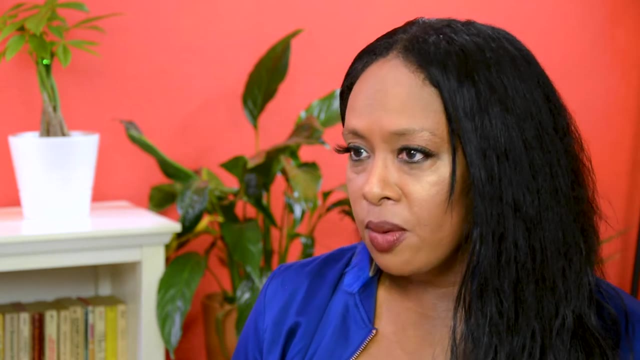 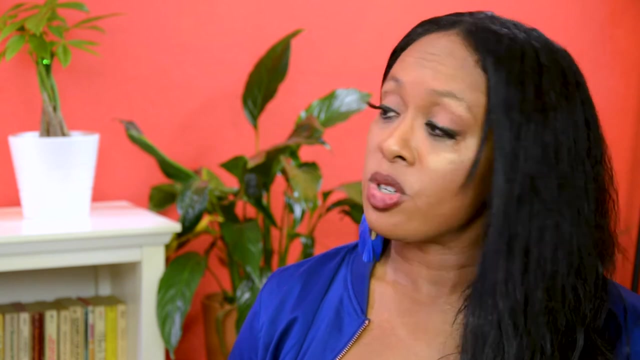 You know you go to my castle in Milan. you will find shelter there, And so she's such a powerful figure to me, From the quintessential rags to riches story, where I will not accept you not letting me in this door. I will bust open a door somewhere else. 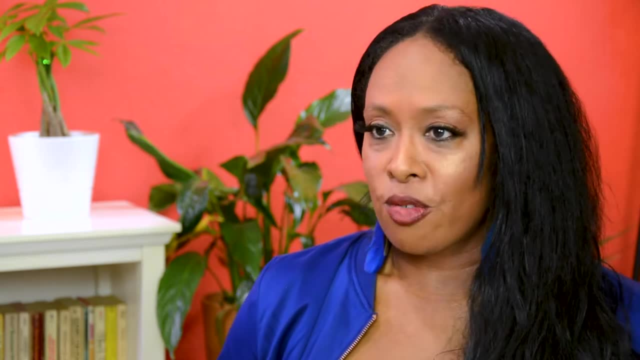 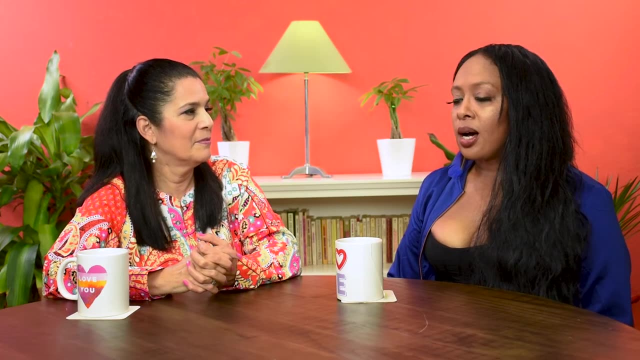 And that's so beautiful to me And so vivacious of her And she desegregated so many things. I do a sequence of her in Vegas And so she was a huge part of the movement. Now I have the civil rights, the civil rights movement now. 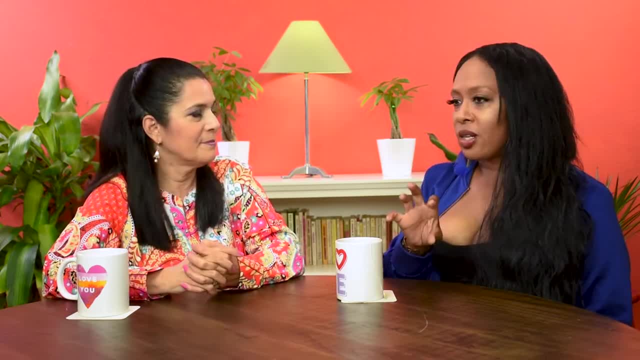 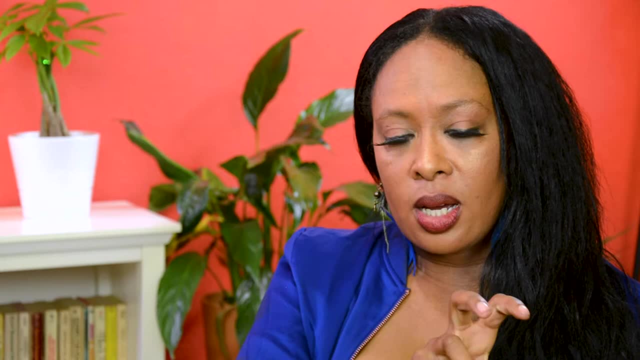 I have her in the civil rights movement, The civil rights movement. Now I have her in the civil rights movement, the center, and you know you guys are going to image. you know I have her in the center and I have all of the other women around her. what's interesting is each woman. uh, I was trying to. I 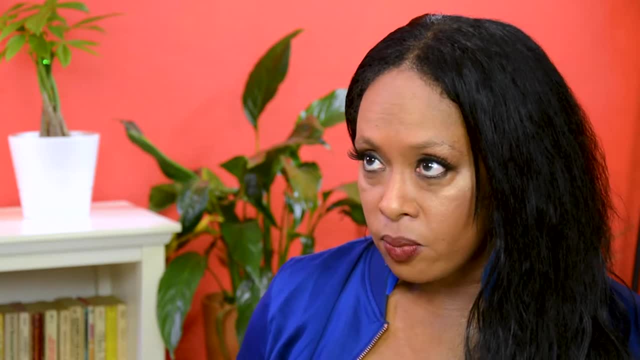 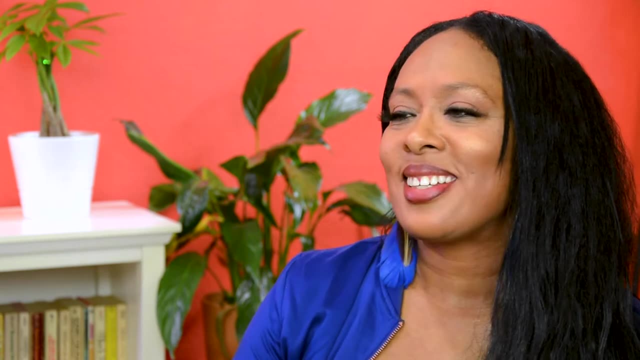 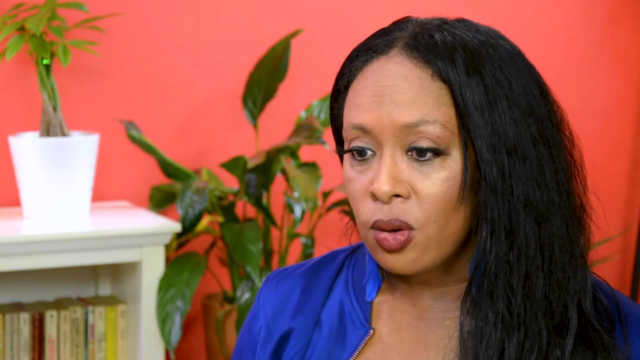 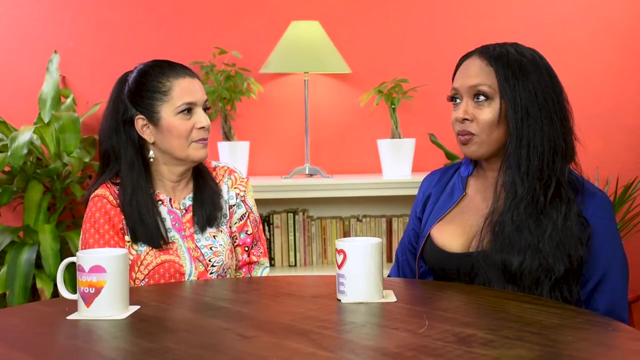 recreated their iconic- look yeah, iconic- image, imagery that we have of them. and when I did that, um, I remember one of the first theaters that I had it at theater, theater on Pico in Los Angeles, I had it as a giant nine uh six by nine poster banner rather, and I mentioned that because 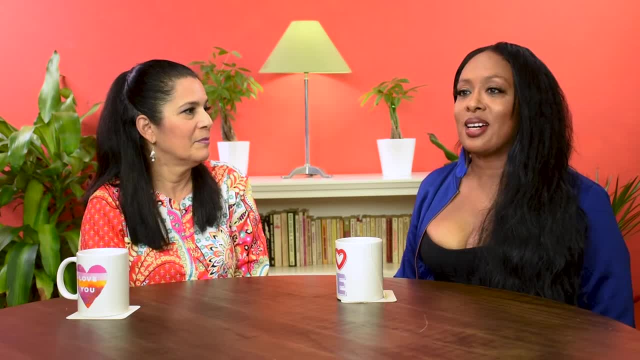 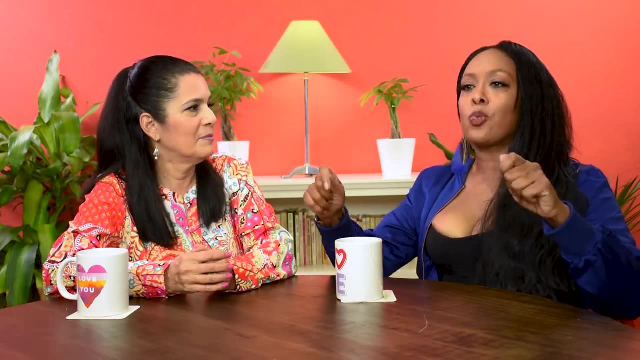 this woman and her children were walking by and the uh owner director there, Jeff Murray, a great actor and director in his own right- he said I because he had literally just put it up and was checking the level of it to see the, the size, the angle of it- and this woman and her children came. 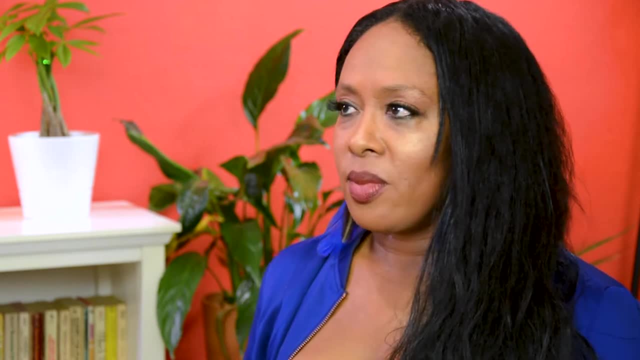 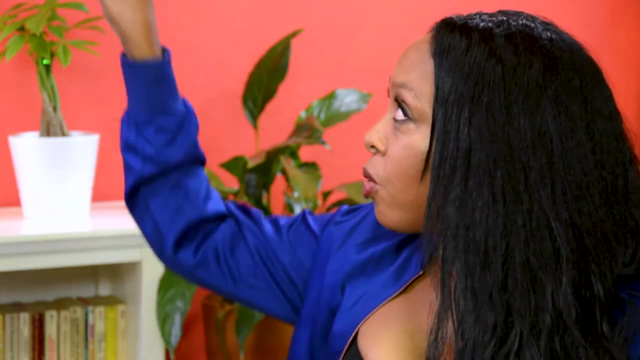 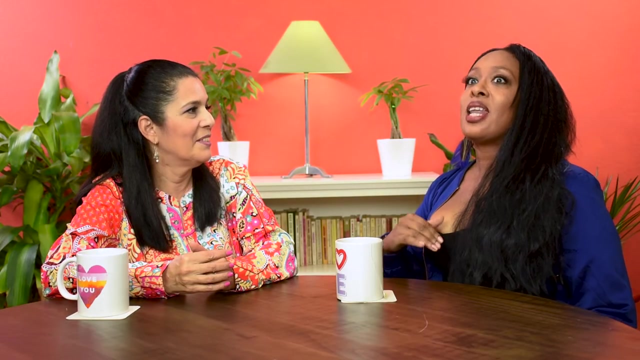 by and walked by it and and and um, they walked by it and the woman did a double take and then she stepped back and she started pointing to each of the women and explaining it to the two children. and in that move me, because I said before they. 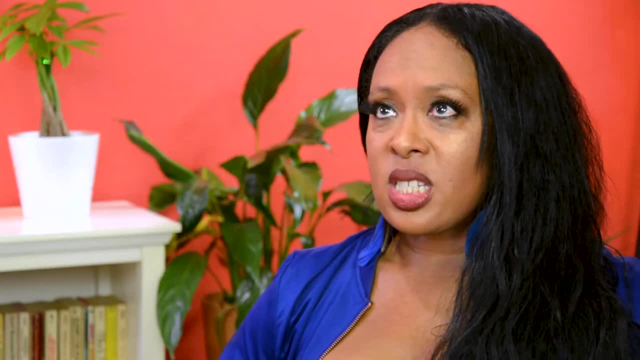 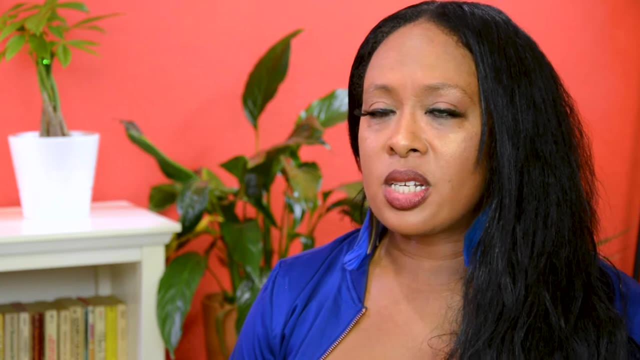 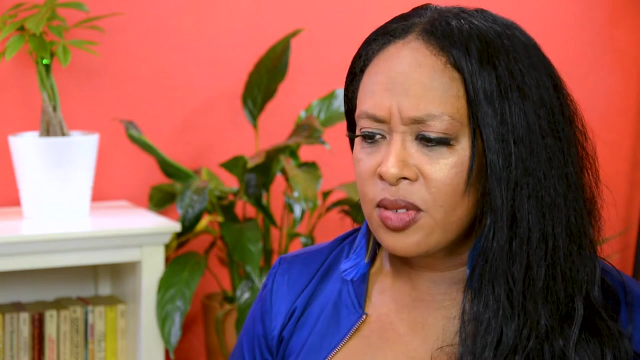 even see the show. you know it's teaching people and so I I feel like it's outside of me. the way in which I've presented this is on a on a different level than I've ever experienced it and, uh, the audience has been amazing and uplifting and spiritual and and people get a feeling from it. 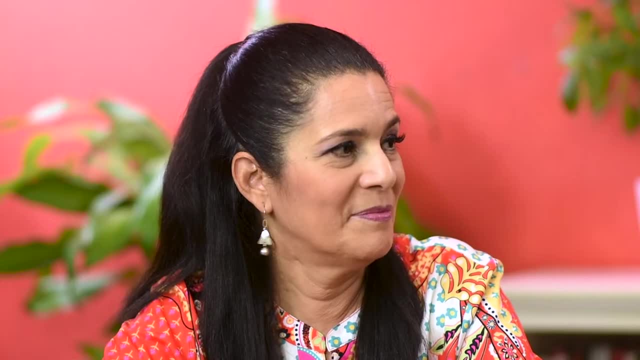 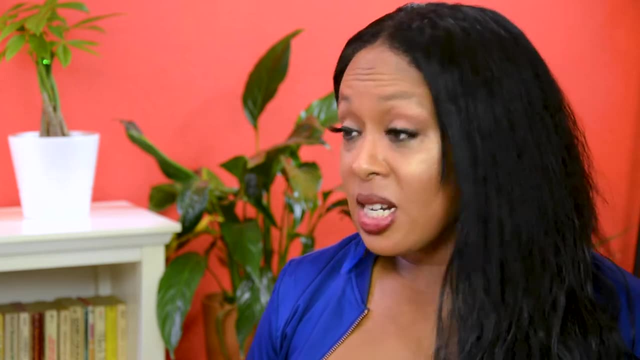 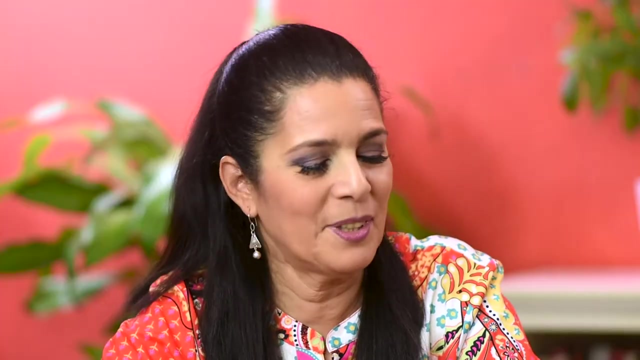 uh, very much like a gospel play, without it being overtly a gospel production. but there's a, there's a spiritual feeling that people have, um, and it doesn't matter, it's not just quote-unquote- for for uh people of color, for uh African-Americans, right, right, it's, it's, it's it, but it's, it's. 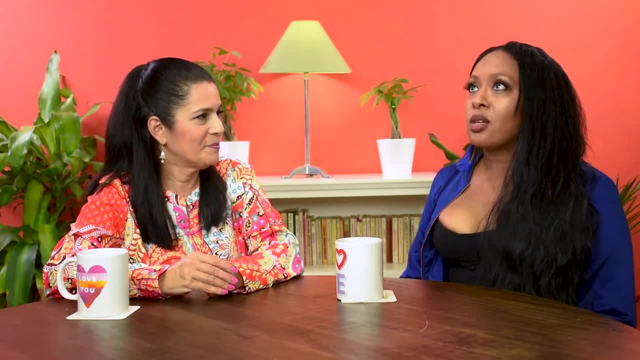 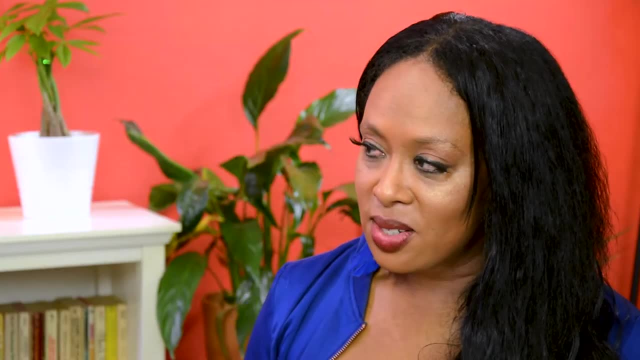 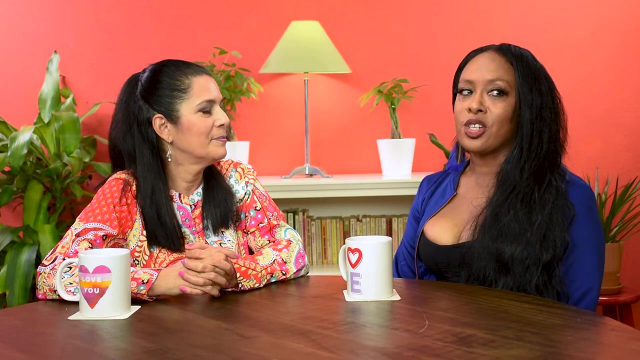 beyond that, it also speaks of an underdog situation and surviving and, uh, thriving and overcoming that people respond to. and can I share a little side story regarding the banner? okay, so as artists, and often with theater, we're very limited on budget, and so we. that's how you're often able to be so creative, because you don't have the budget to do things. 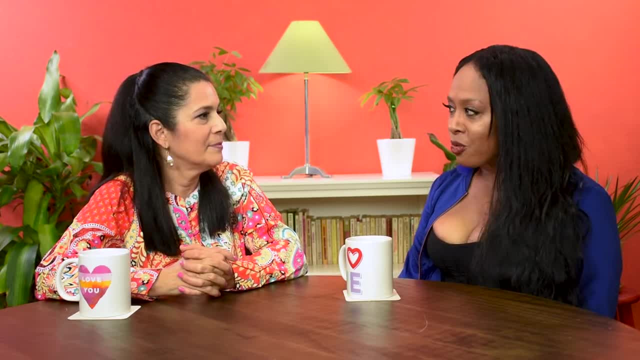 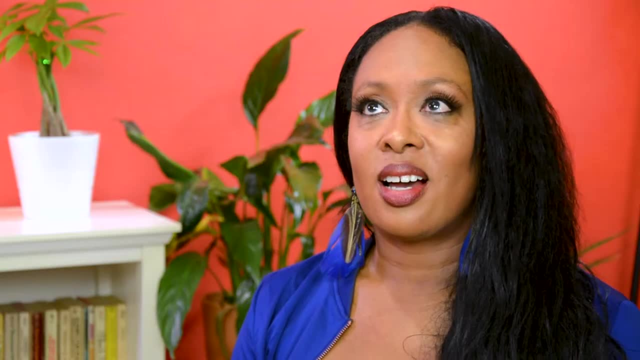 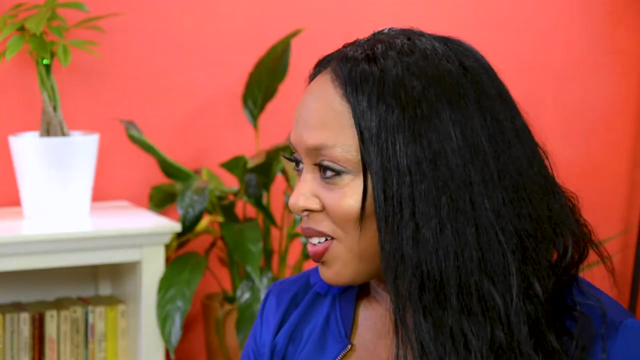 on on a main level. that was my publicity. that big nine foot poster that people drive by on the street. that was my publicity push. and one day, uh, came to the theater and the banner was gone. what the banner was gone. I was like it was it was. it disappeared and no one. 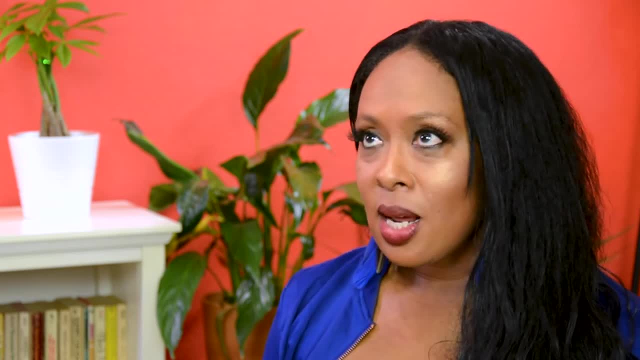 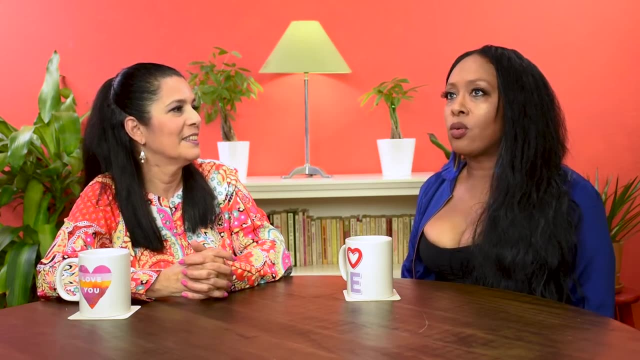 knew what happened and went over to it and I was devastated. I looked over at it and it wasn't like it was just ripped off because I looked, I looked in trash cans, I look, I was like somebody, just you know, vandalized it and we looked, and when we looked at the rivets on which it was put on, 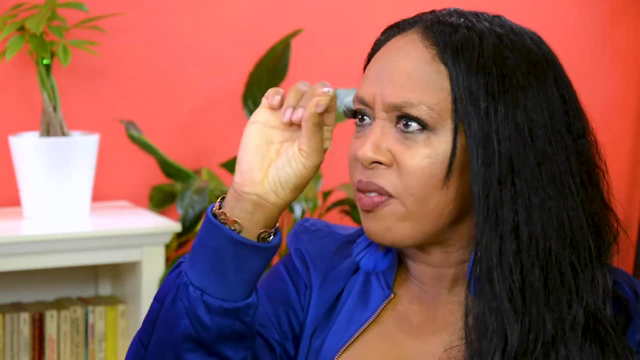 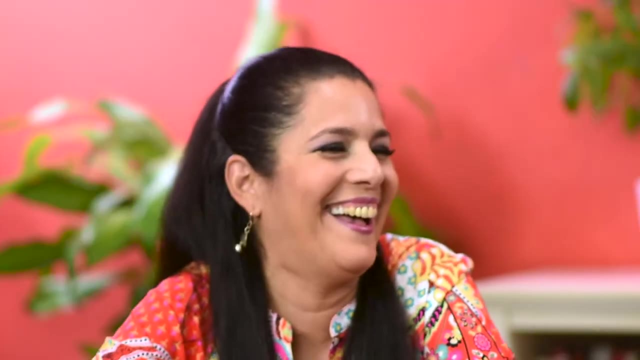 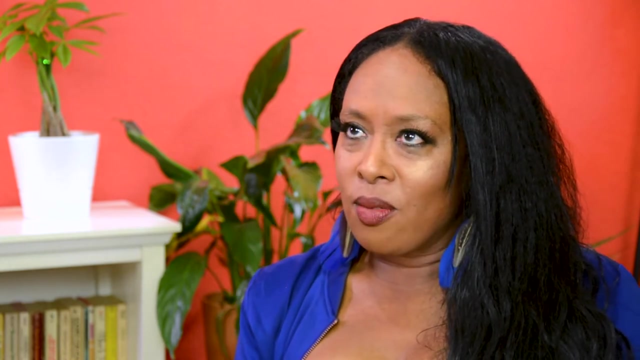 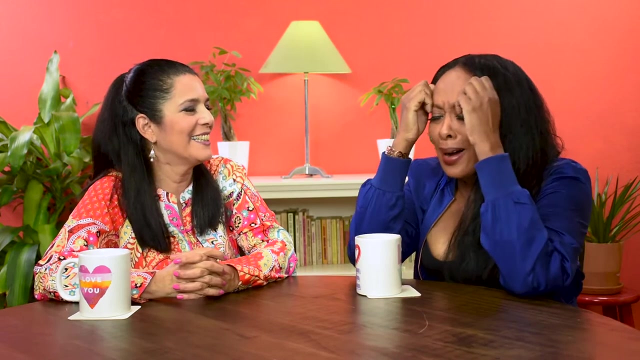 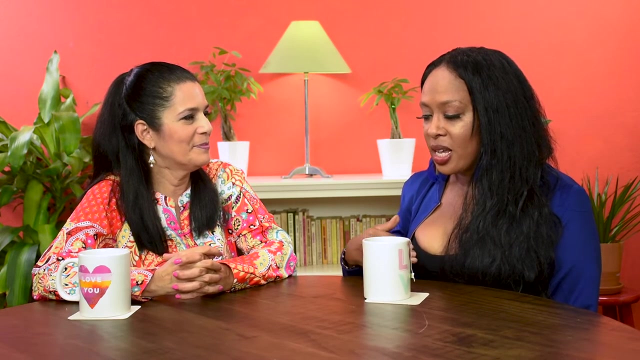 carefully cut around the rivets and I'm like somebody's sitting at home with the beer. oh yes, it was a. it was a fine blend of um, um, uh, flattery and also creepiness. you know, it's like somebody. so um, yeah, so that did enough, but but there were so many things that had happened along the way in. 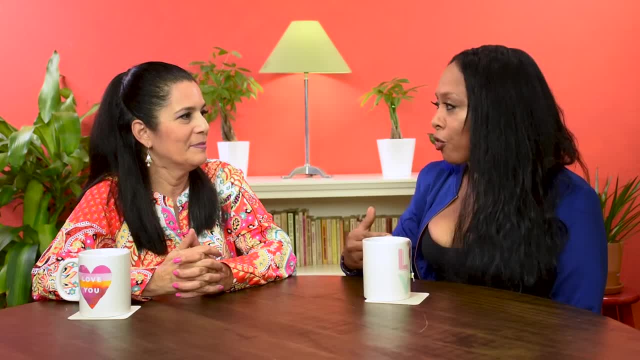 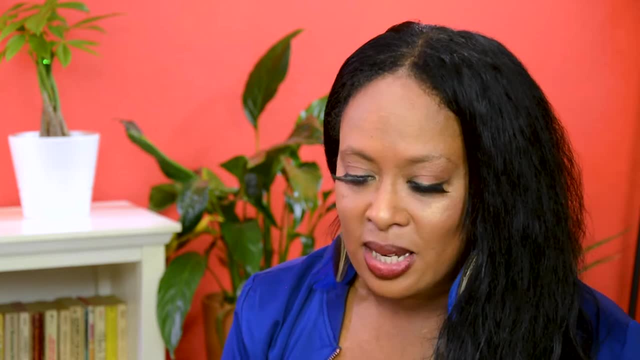 the production and living this to, to bring the show to fruition- that my cousin told me something, my cousin Charles Holman, who was an actor in its own right- may he rest in peace. it was so supportive of this and he said to me: Sandy, you can't expect to play women who've gone through. 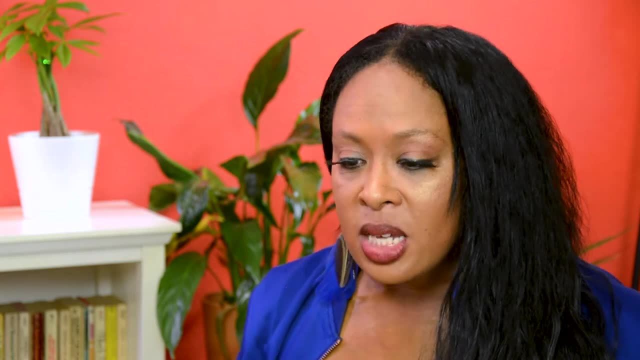 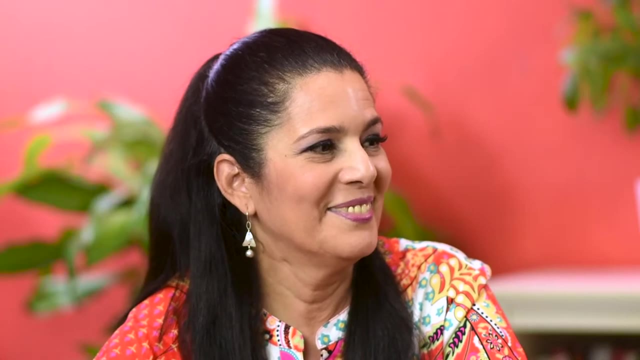 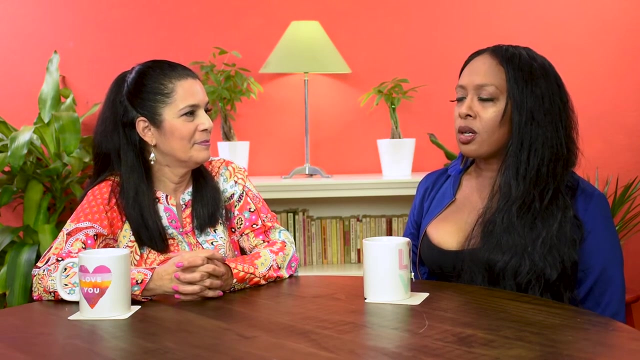 so much, without being in a pool of things that you need to overcome, to bring them forth. you've got me there, you know, and, and and to do them honor. so there's, there's, there's, uh, there's a lot that I've learned along the journey, even when I was writing it. 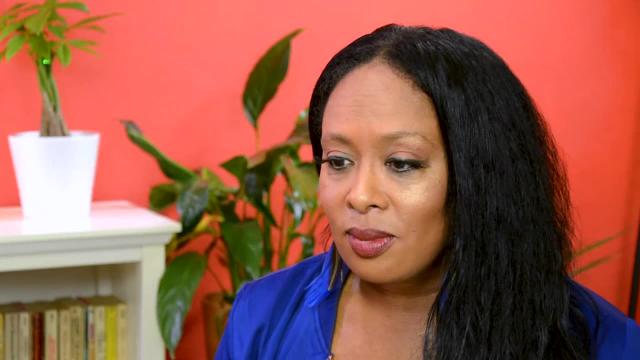 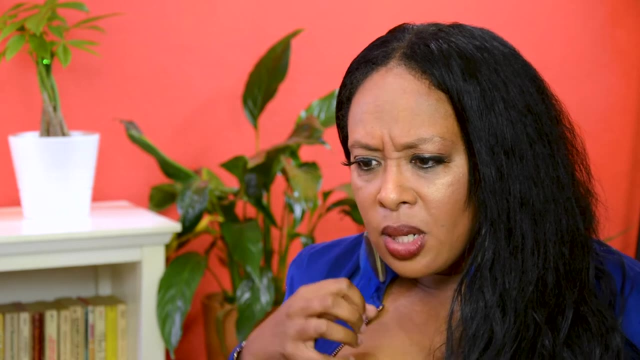 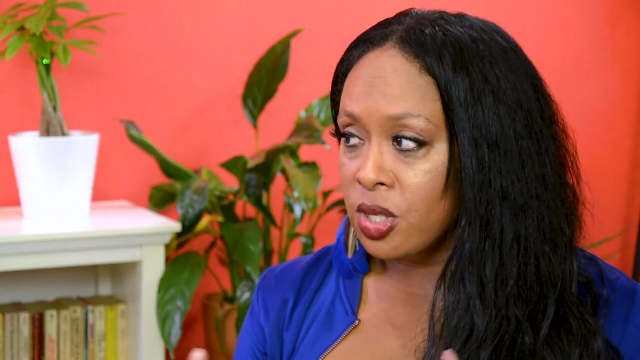 I didn't know, um, I I at first I was thinking I'm getting, I'm getting the details of it, but I wanted to get the the humanity of it, beyond just the legend of it, but the human response and what they were feeling and, uh, that everyone can relate to and that's what's universal is that when people 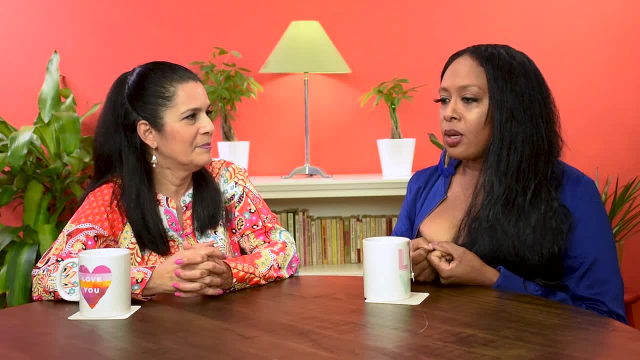 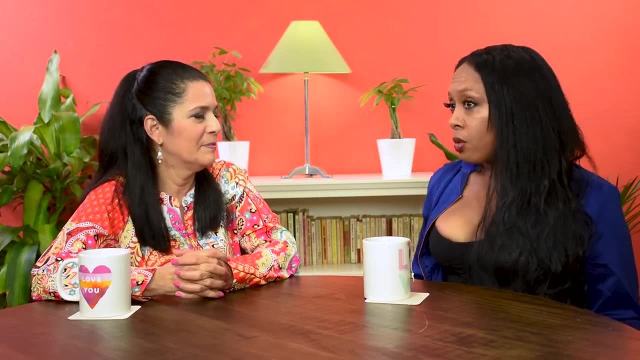 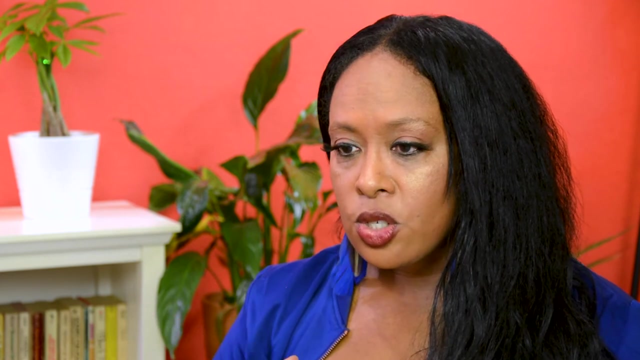 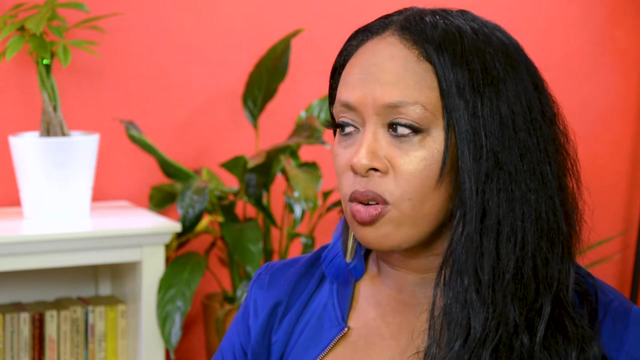 see it and the reactions, and you'll see some of those um, uh, it's that they realize that it's not that these were just super human people, super heroes, you know, doing whatever. it was the average person and that, and, and their, their situation, where it came to a point where they could make a decision to make change, be the change or influence the. 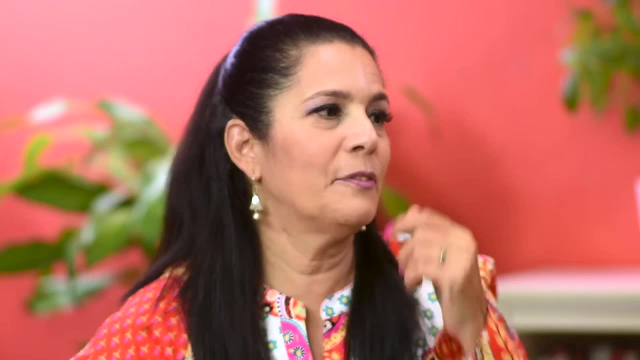 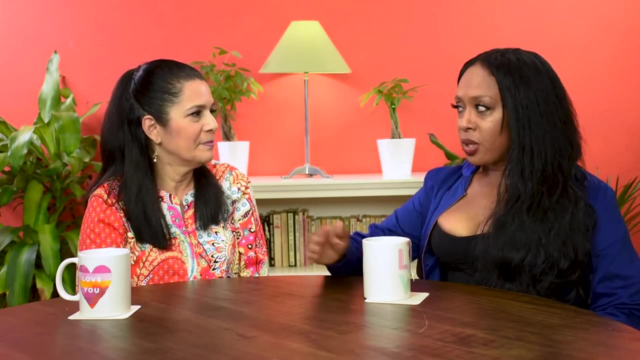 change. they didn't want to turn around and they stepped up. and that's what you are saying, that's what you see in the show at that moment and people you know it speaks to them. that's what they relay back to me. um, there are people that have seen 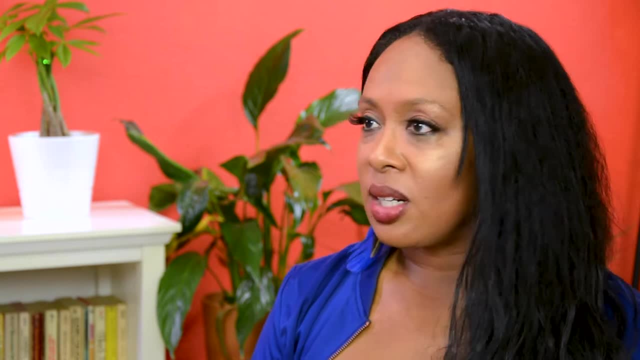 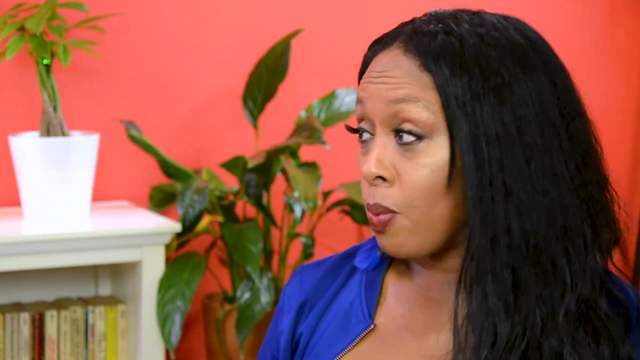 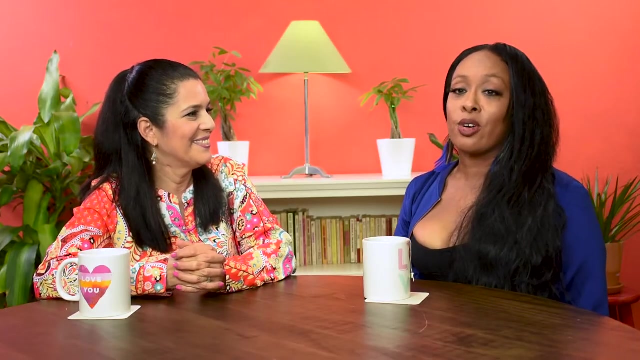 that are saying, um, i feel deprived. i didn't learn this in school, and there's people that come and see it over and over again and that blows my mind too. um, there was, there were some people who it was that theater? theater is right near roscoe's chicken and waffles. they brought a. 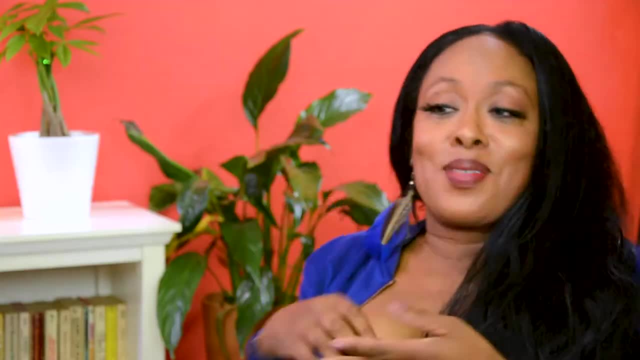 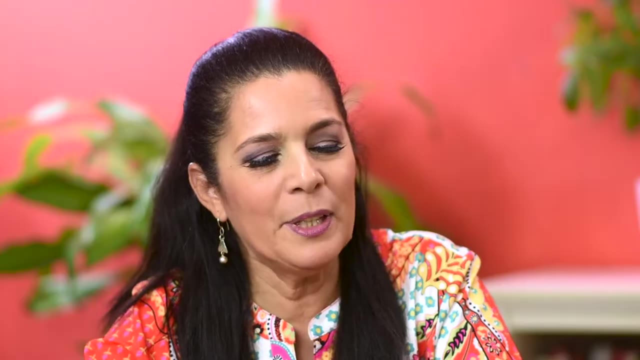 chicken dinner up there on the upper rafters and they were sitting there and it was like they turned into dinner theater and they were like this is my thing, this is my you know, and i'm like, so that tickled me, doing it in los angeles and then taking it up to the bay area. 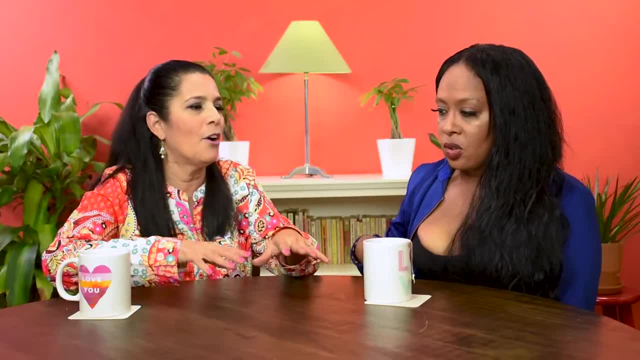 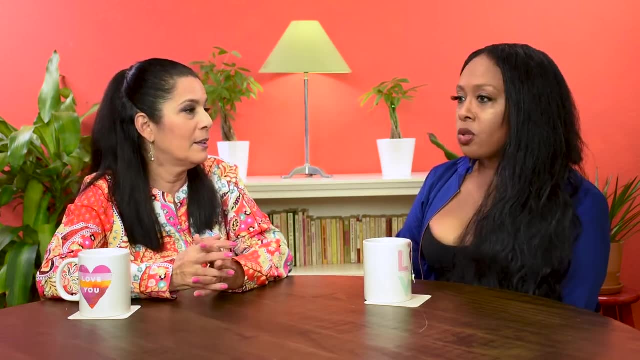 to do it. what was the difference of the audience? because i i would assume that there is such a different audience in the bay area. well, i went to school in the bay area at uc, berkeley, and that- i will just say this would be honest- it's a more literate community. i mean, they're more tapped in. 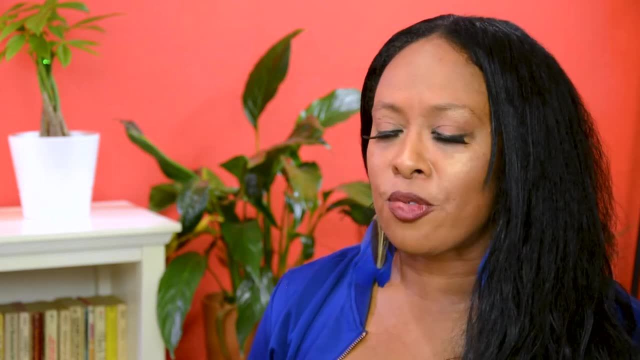 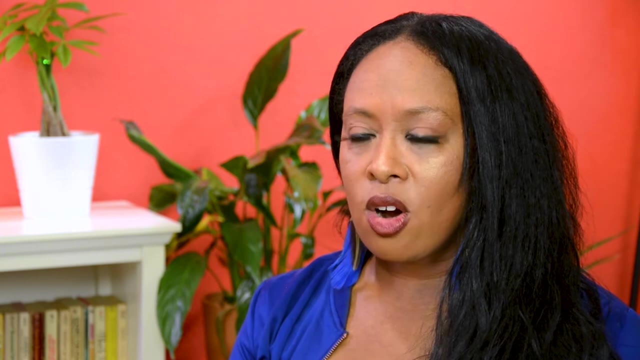 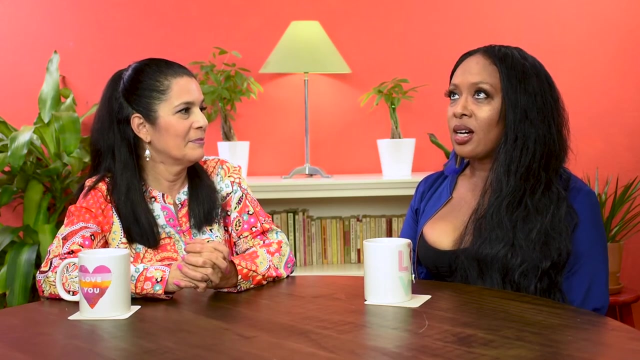 it's the, you know uh, foundation of the black panthers and all these different organizations where, um, and they're more tapped in uh than they are out here. so, um, there's a, there's a richness to their appreciation too, and, uh, to get history teachers that are like 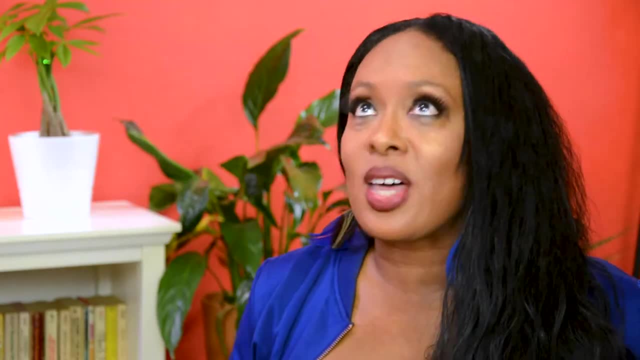 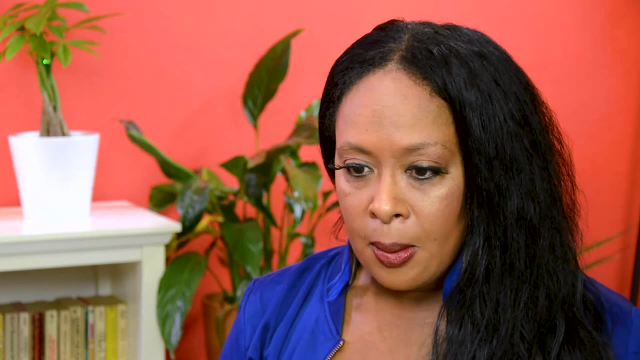 you bringing stuff in that i didn't even know. you know what i mean that. so that was. that moves me to the respect for, for the craft in terms of the writing. this is the thing also with this project that it allowed me to step forward and and it's, it's. 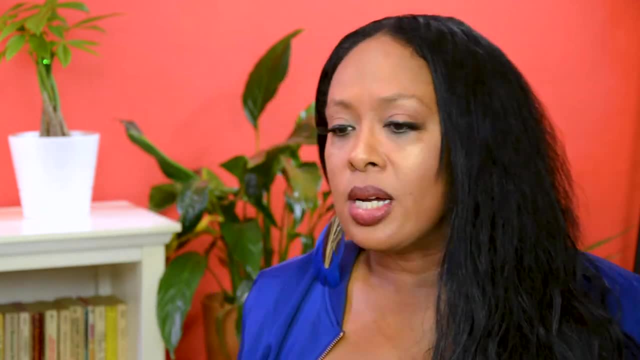 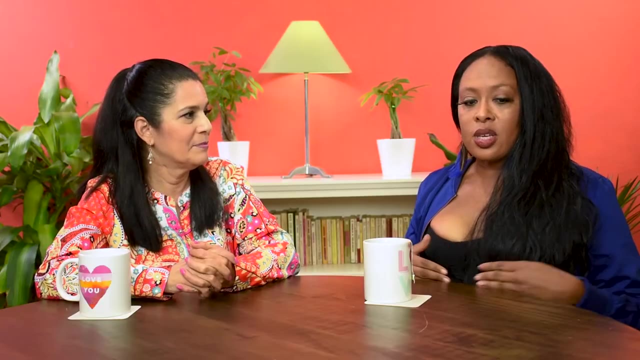 i'm jumping into a lot of different things. there's a lot. there's a lot that goes into it, but this particular project came at a time when things had gotten slow for me as an actress and i think a lot of the onset of reality tv has affected a lot of us seasoned actresses that have lots of credits. 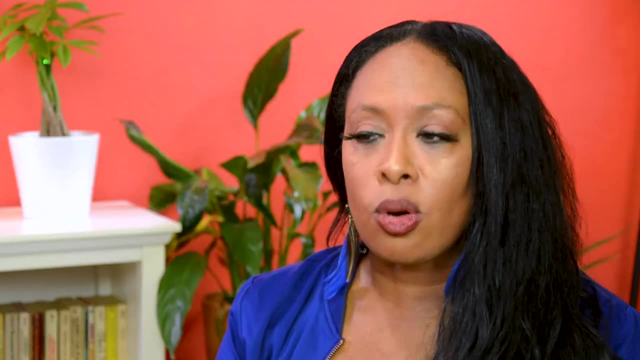 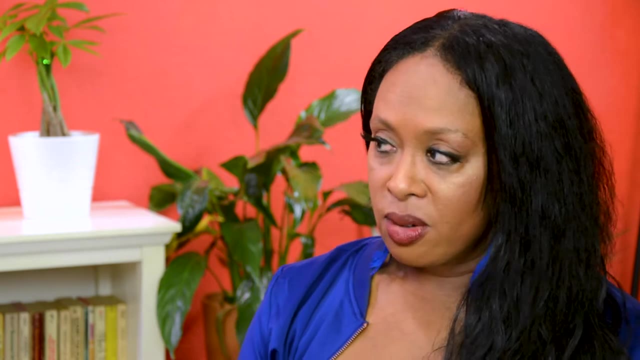 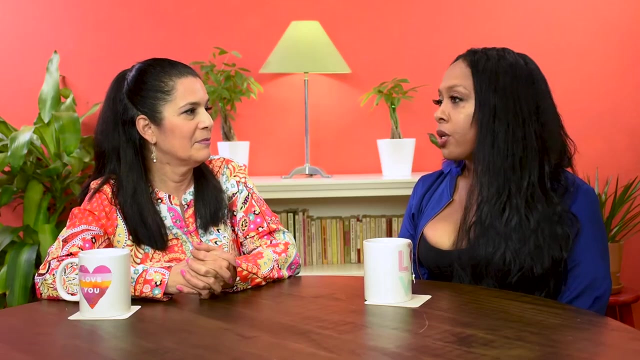 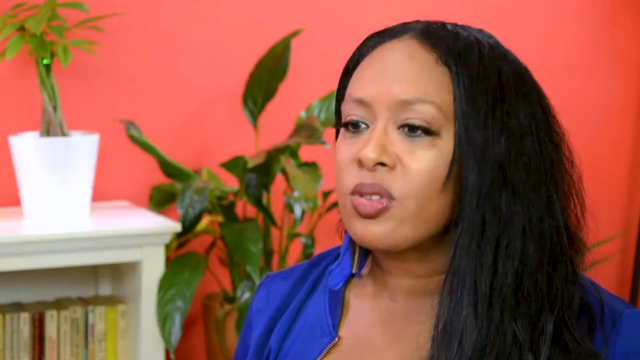 and things like that. this show allowed me to write direct produce and uh, characters that i may have never likely been cast in um during the time that i ran this show, over 200 performances. over 7 000 people have seen the show. during that time of doing that, i don't think i've ever felt more creatively fulfilled. 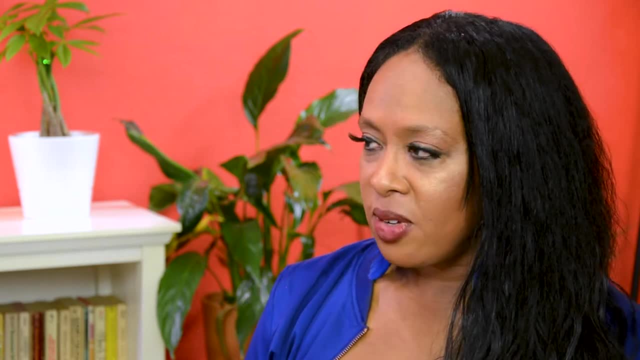 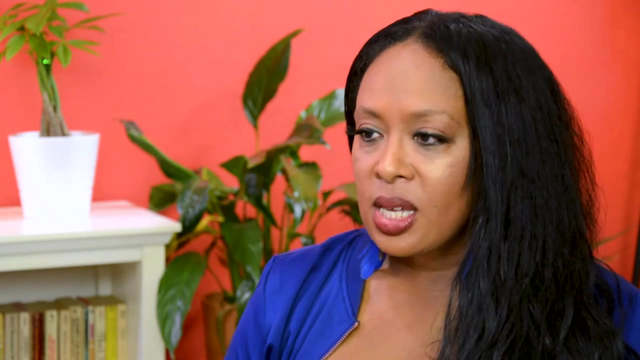 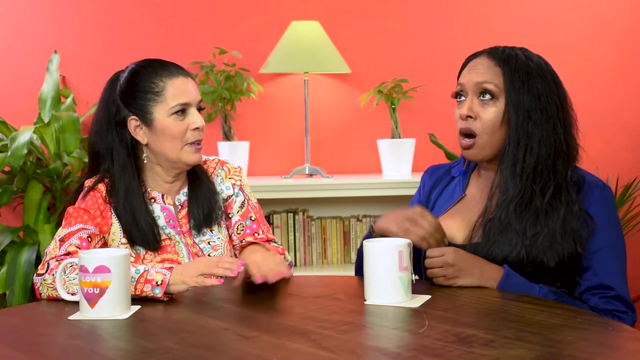 you know, um, as fun and wonderful as film and tv stand-up. all of that for being able to create this every night and take that audience on that long journey of something. it was so rich because each of the women into a different aspect of you, you know, not just as an artist, let me. let me jump in here because 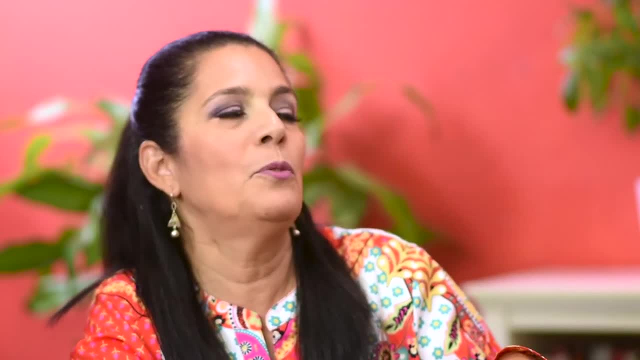 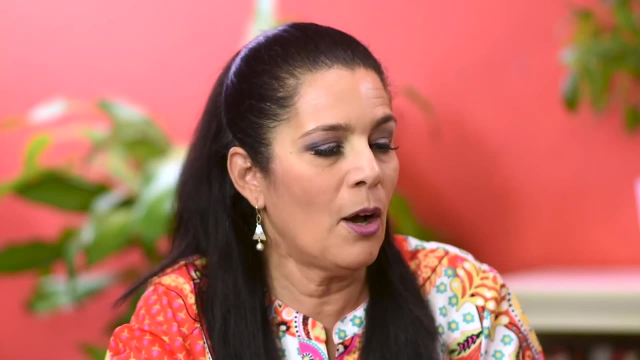 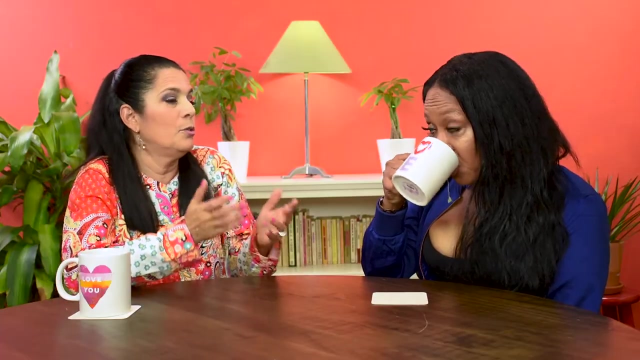 yeah, i think what the audience has to know is, first of all, you have been doing sketches for a bazillion years, yeah, between sketches and stand up, and so you already had a sense of character, because in your comedy, you, you do a lot of characters. yes, you, you bring them into the party. 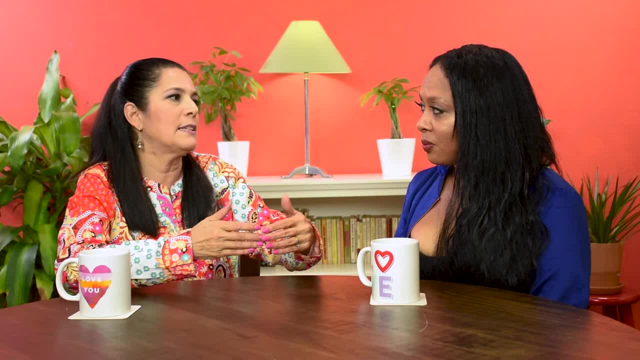 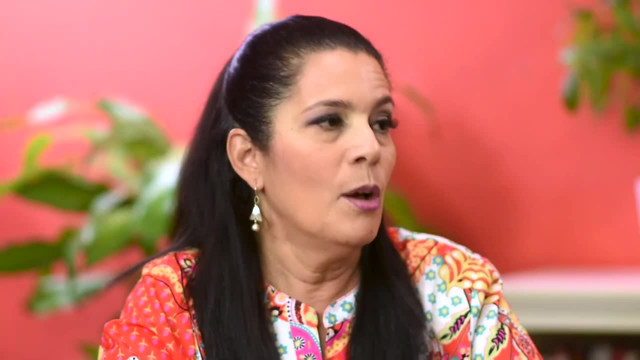 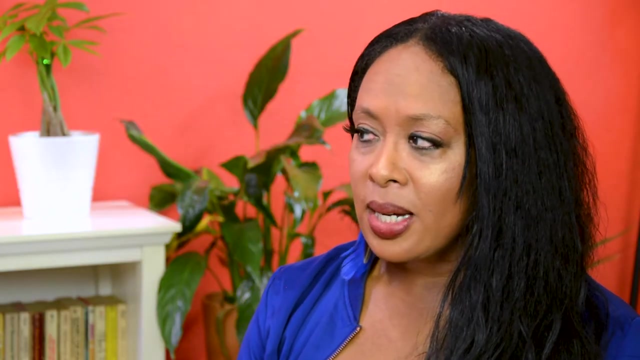 so that this was an extension of something you were already doing. i mean, you were already writing, you were already creating characters, but now you went into another zone. yeah, i had taken it to another level and i'm known for my comedy. um, i'll get people that may not know my name, but they know. 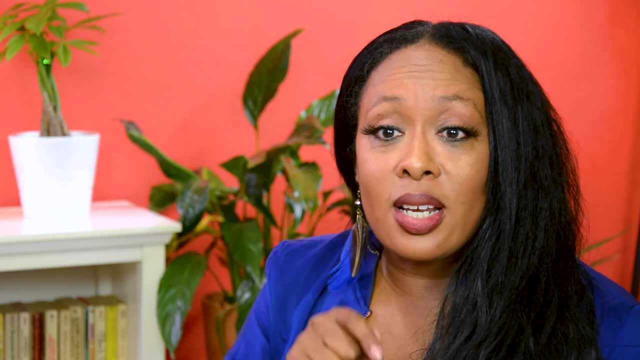 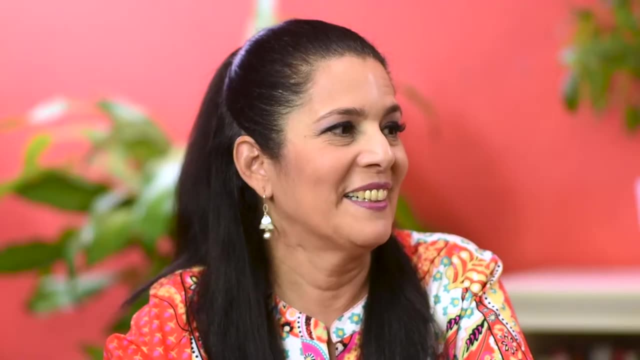 my work and they're like: you're that girl, what's that show that you? you're on that show, what's that show that you play that that crazy woman on? i'm in the neurotic one, i'm like all of that. that's what i've been, you know, kind of typecast as and um, when you do this, you get to. 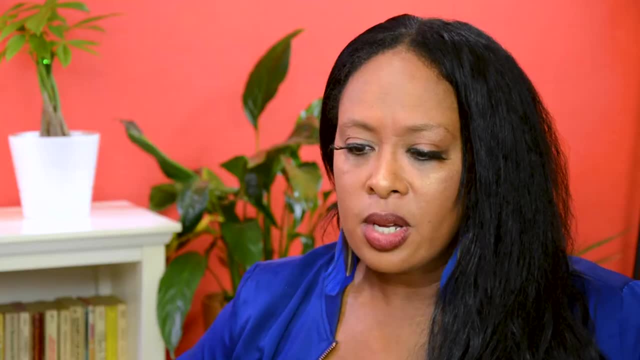 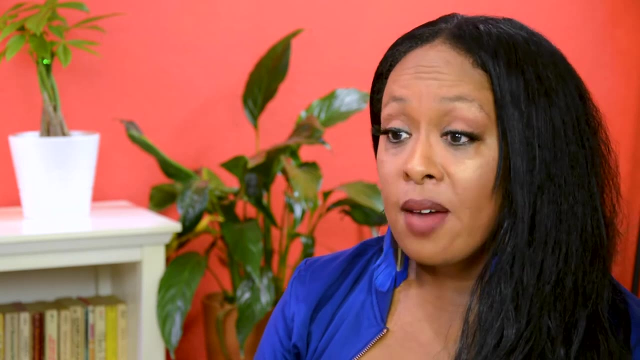 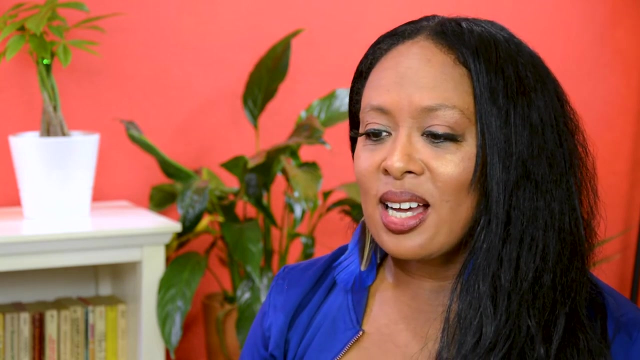 work all of these other muscles. when you have mentioned uh phyllis wheatley uh, who is an iconic uh writer, pioneer of african-american literature, um, when i i wanted to get such authenticity with the characters that i know her background: she's from senegal, gambia, and brought here on a slave. 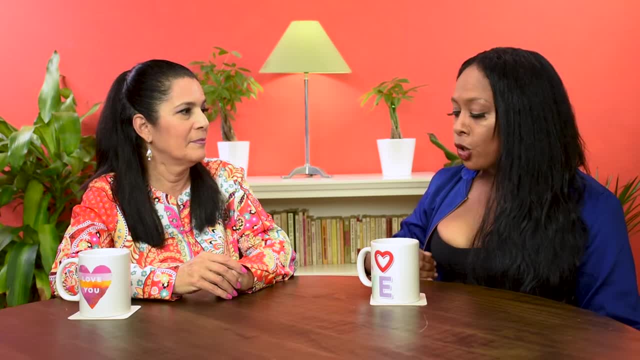 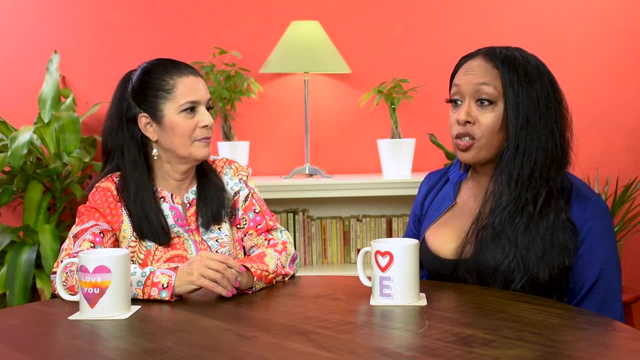 ship and i would want the specificity that we would learn uh in, uh, larry moss's class. larry moss is an acting teacher here in los angeles. um, uh, extraordinaire, and whenever somebody i knew was going to uh africa, or a friend of mine, i would say if, oh, if. 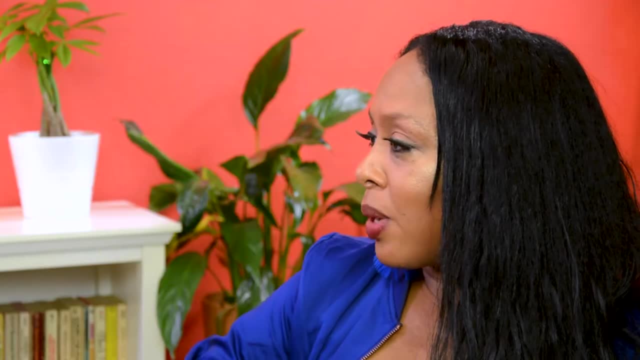 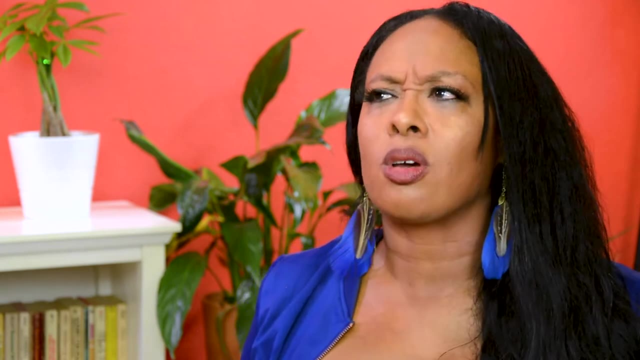 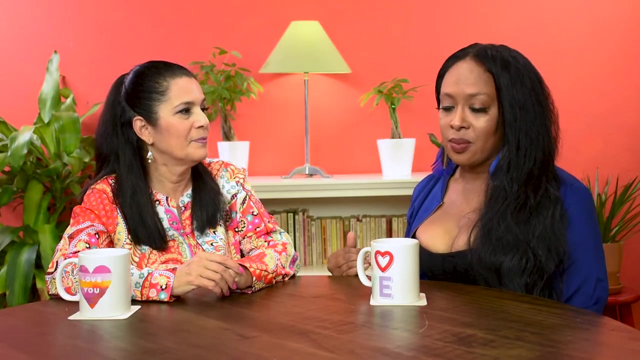 you're going to mali or senegal, gambia? um, just bring me back a pebble so i can sew that into the dress, something from her home from her home, something that is hers, that is of her. that when i was going out there, and what's interesting is is over this time i've found out, i've done the, the dna. 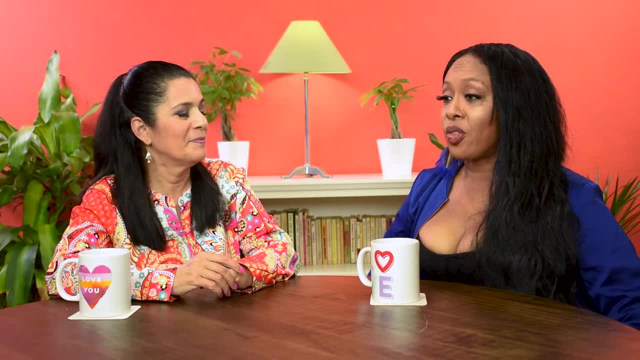 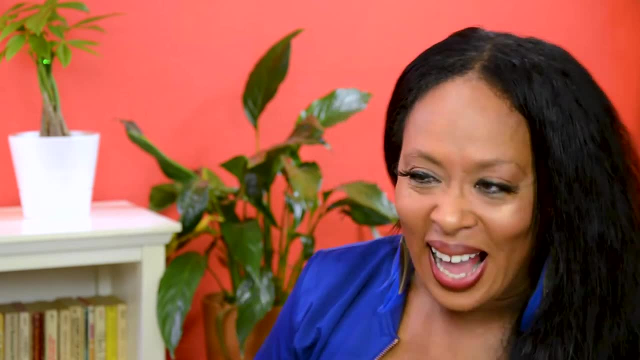 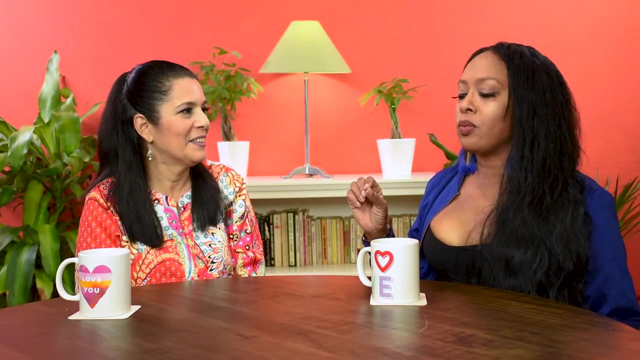 and that's one of the things that, and, uh, with all of the surprises that showed up, in that i can be easily offended by just almost anything, which i love, i love, i love that i can tap in and that i'm i'm kind of related everybody everywhere, so, um, 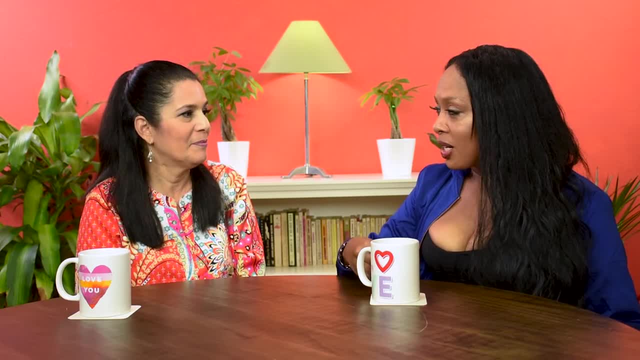 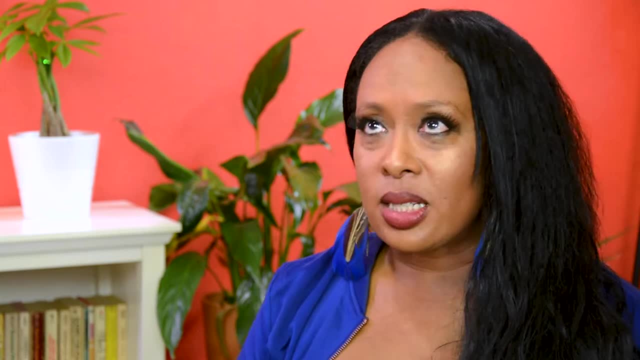 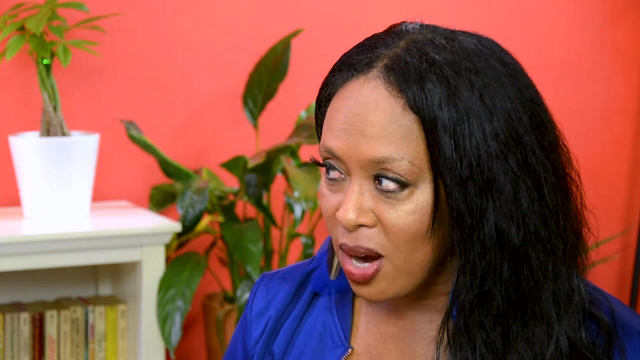 with that I found out that I have that from her region and that just moved me in such a way in terms of it awakens you and we're talking- let's say we're talking a little bit more about the craft itself When we have studied under Larry Moss in his book Intent. 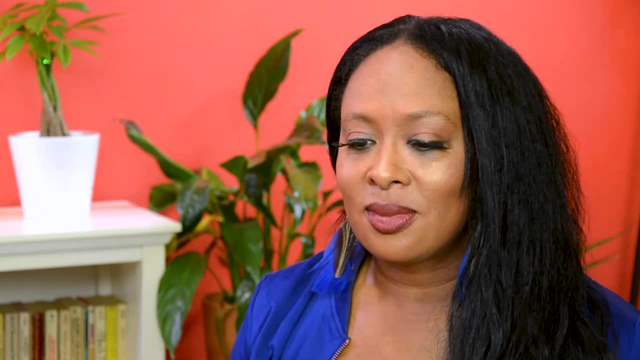 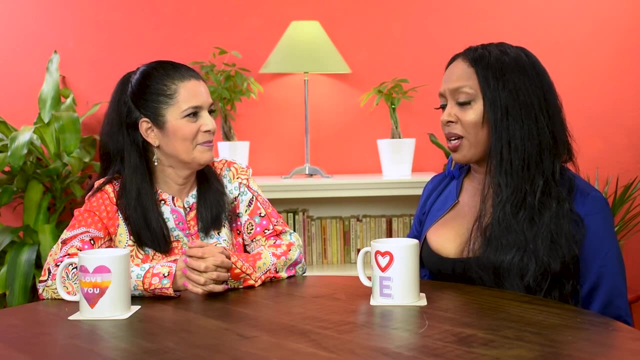 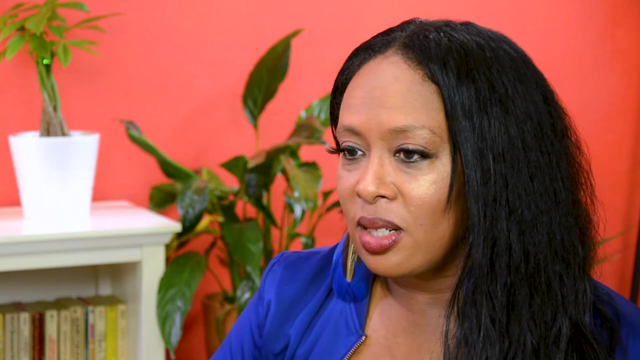 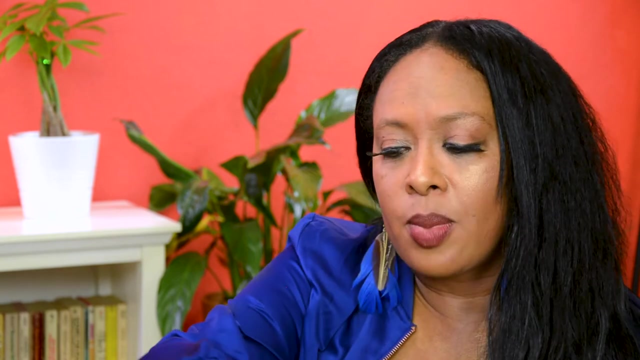 to Live. he would say in class: how you do anything is how you do everything. And I'm like that's not true And I'm like it is, you know, And I'm learning with this show, completion of creativity and going deeper, And it forced me to dust off all of my aspects. 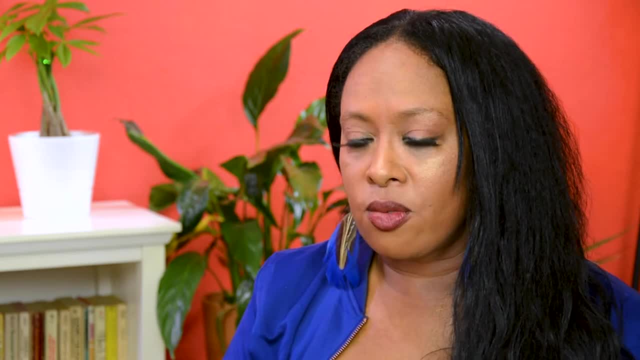 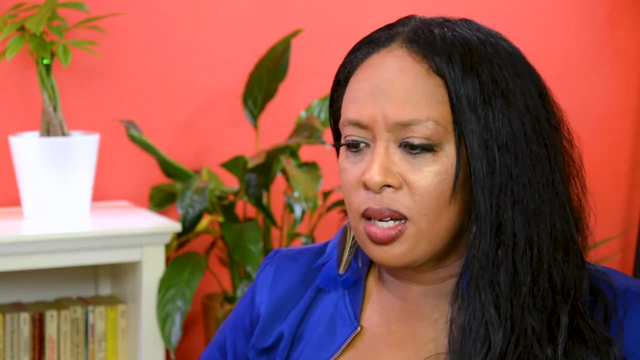 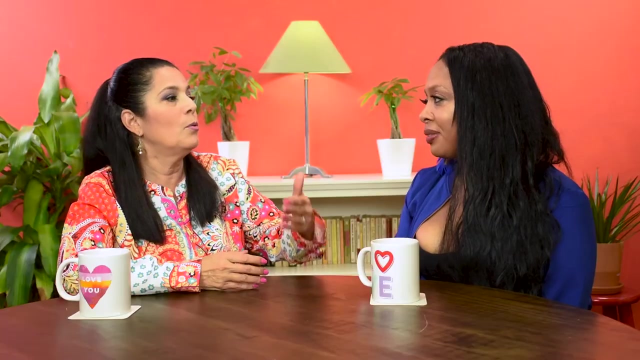 of my creativity into this one thing, to bring it forth, And it has blessed me. It continues to bless me and others, And so it's the definition of a capture piece. Let me ask you, as an African American woman who is hypersensitive, but once you started, 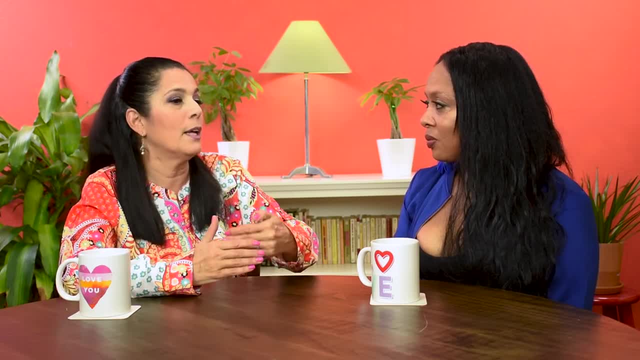 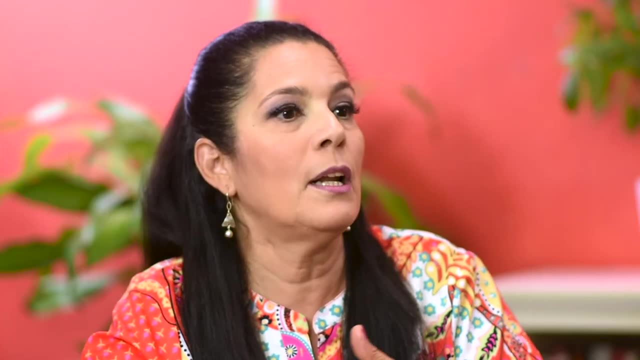 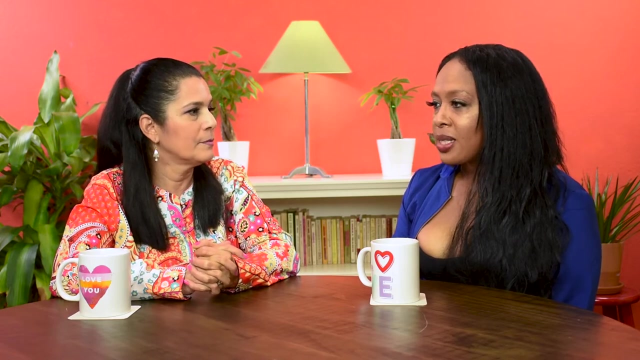 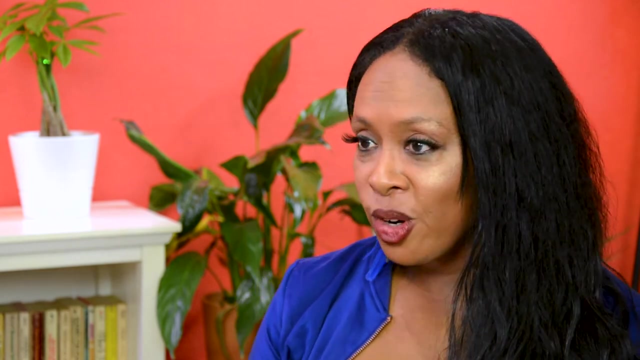 digging in to these women of history and really finding out more about them. how has that affected you in how you look at stuff? now I'm more so than hypersensitive- hyper aware is probably what I'd say- And I understand how I'm able to stand where I stand, you know, and stand in honor of that and to remind others. 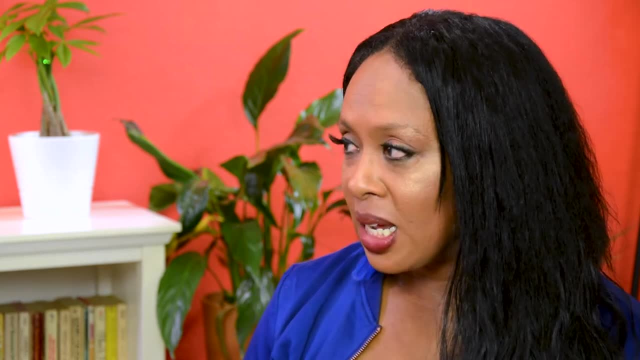 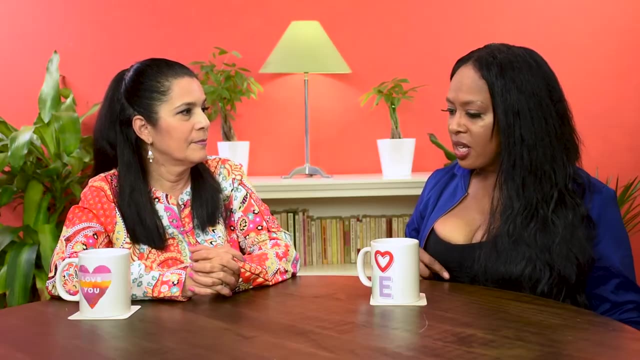 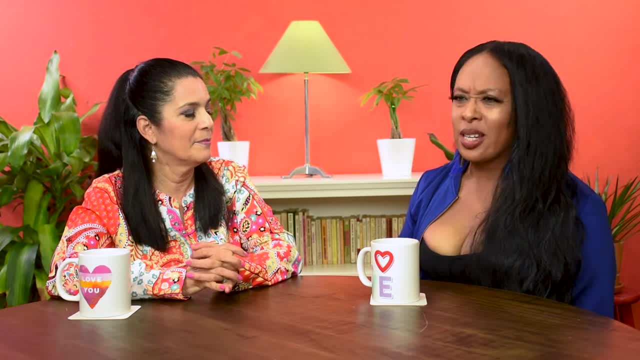 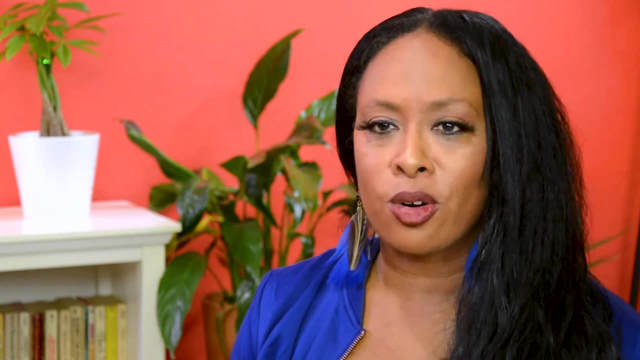 be a part of it. One of the things, one of the characters in Volume 1, I won't say character, but legend of character of Volume 1- is Angela Davis, And when I'm on the megaphone with her at her rallies, and you know, and speaking in terms of 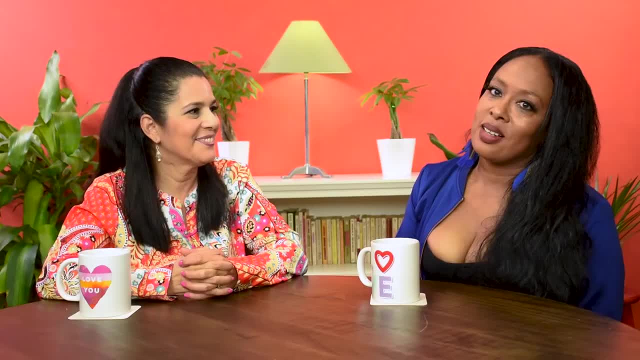 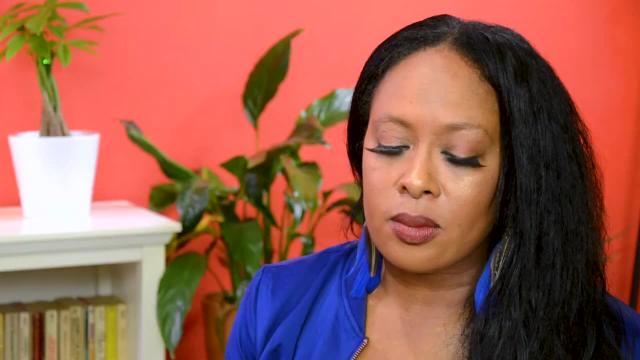 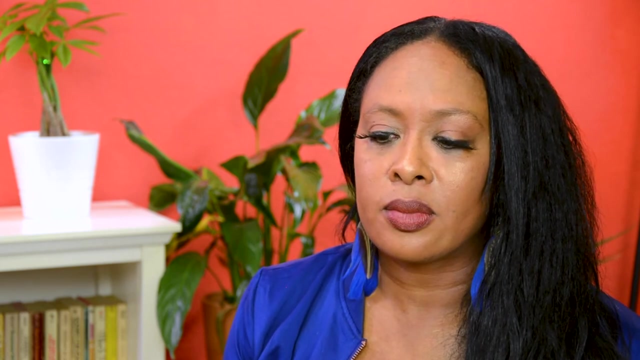 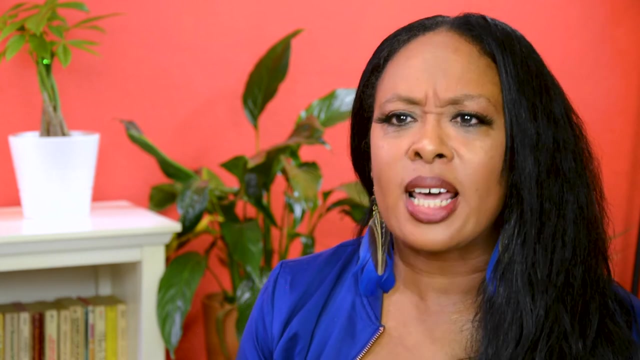 And Angela Davis. Angela Davis Is who Is an iconic professor and civil rights leader. She and and, and and I just you know I'm a women's uh study pioneer and prison study pioneer- um speaking with her through the megaphone and 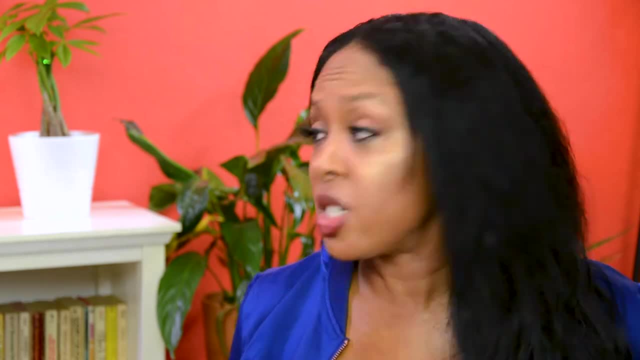 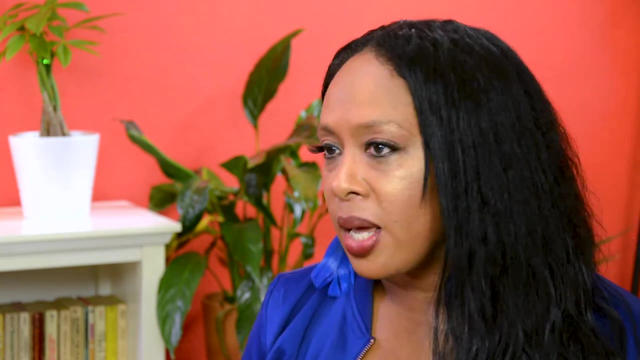 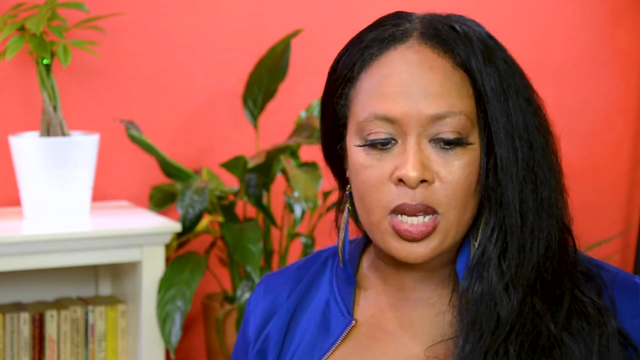 the audience and one of the things that i'm taking you into a 60s rally, as as angela davis, and saying you know, and, and that women should be paid the same as as men, and you can hear the audience still roar because we're still dealing with that today. you know, and even speaking about 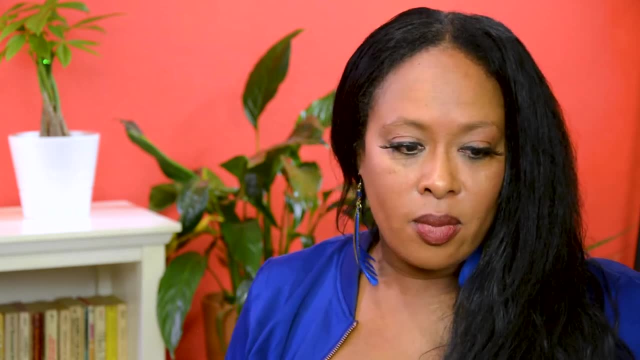 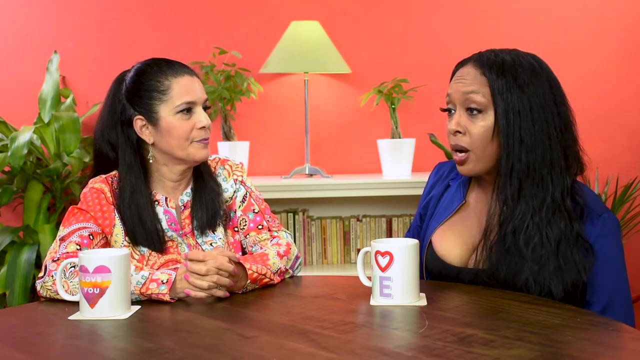 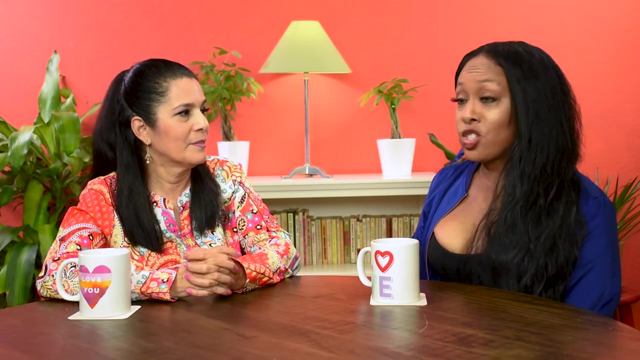 how we arrived at that point, uh, with the history that's behind that. and so i i i'm aware of the connective tissue on stuff and it informs. it informs my writing and performance and a raised eyebrow on stuff that i feel like i'm aware of, stuff that someone may not but needs to know, and 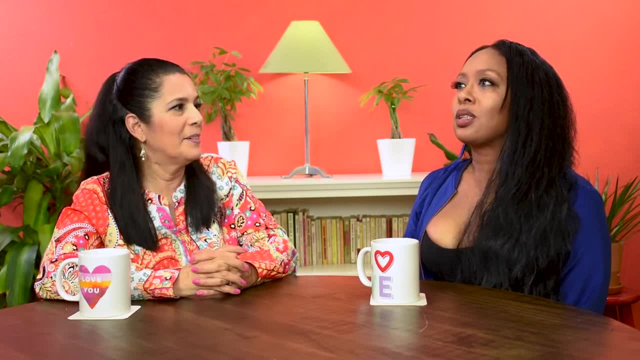 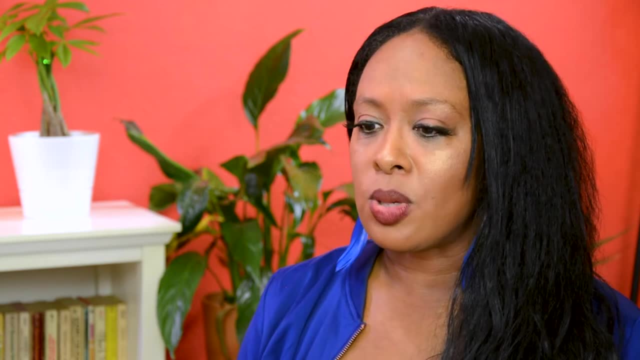 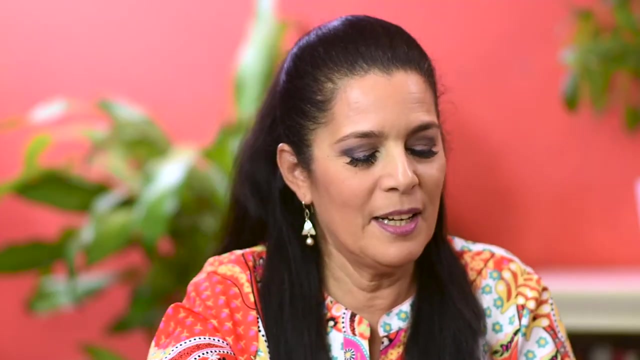 and it's, it's, uh, it's a, it's a, it's, it's an honor, and, uh, that is. my artistic challenge is to be able to present things in a way that that tickle the mind and uplift the soul. so in, in, um, let's talk um shirley. 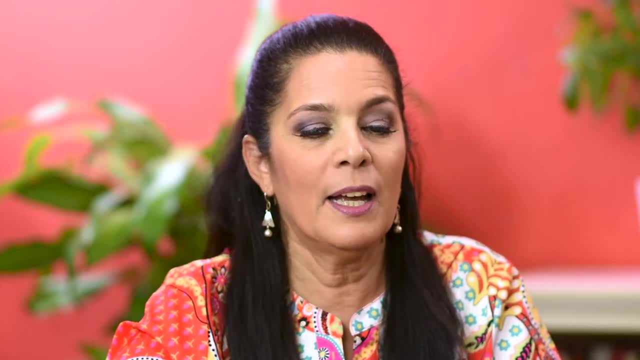 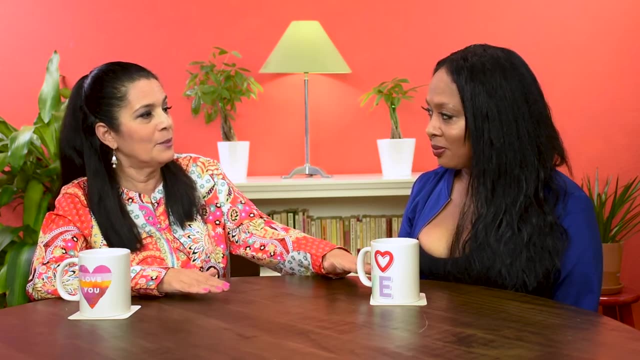 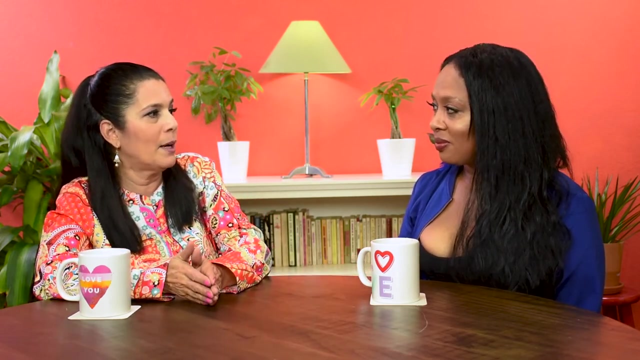 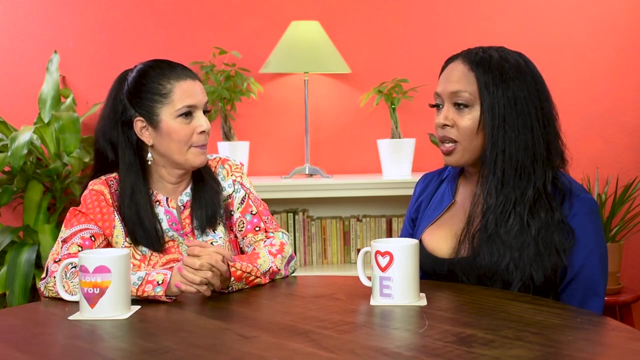 chisholm. uh, shirley chisholm and senator harris. yeah, because the first woman who ran for president was shirley chisholm. and then what? 40 years later, we had a black woman running for president. yeah, that's uh. once again, that's the connective tissue that you see, and and the echoes of that, in fact, when 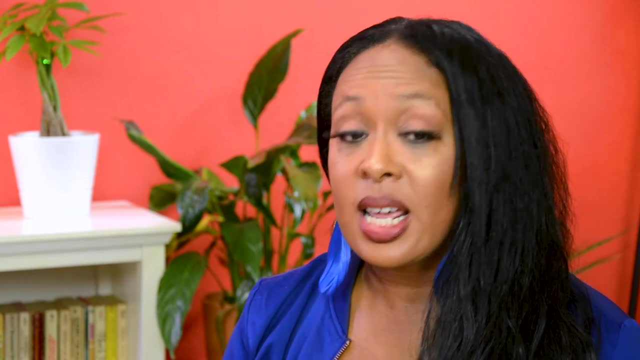 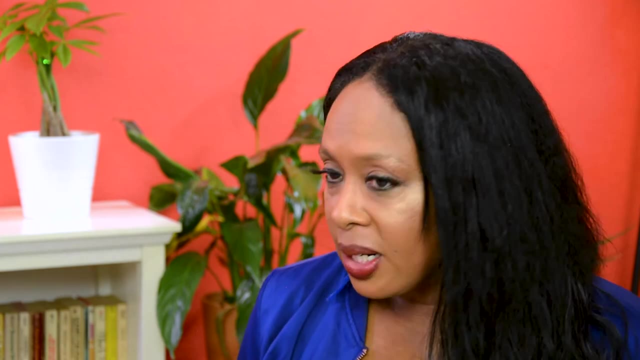 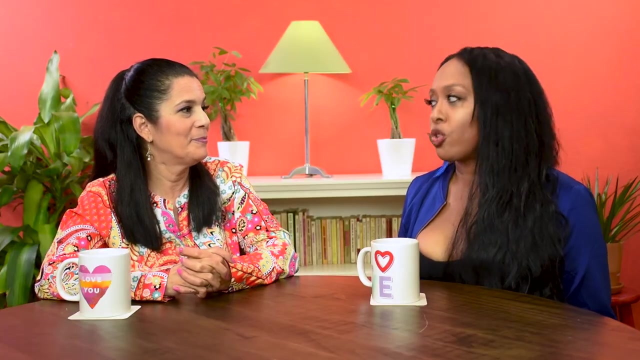 shirley chisholm ran uh for uh, president, and she is someone that i didn't know until i was researching the other way, when i was doing the in-depth study, i was like wait a second, and i'm like i gotta put her in. and uh, shirley chisholm was a badass and, um, people started having t-shirts of her that would. 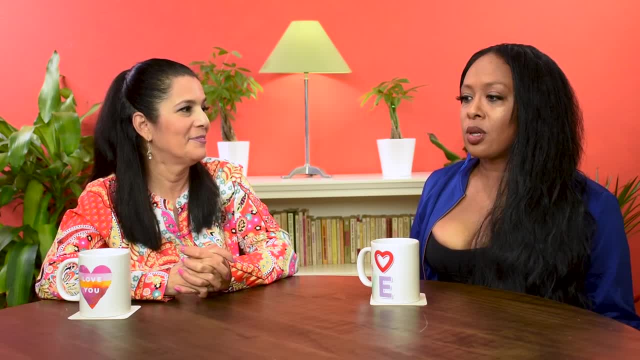 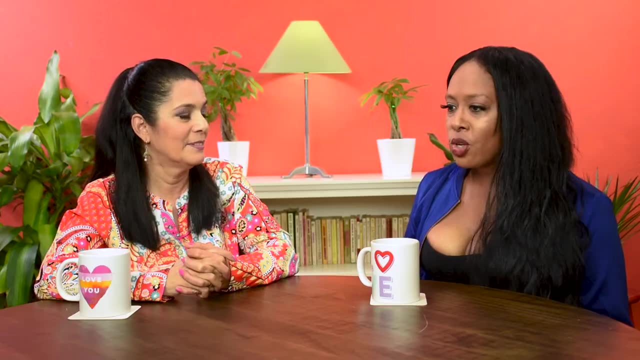 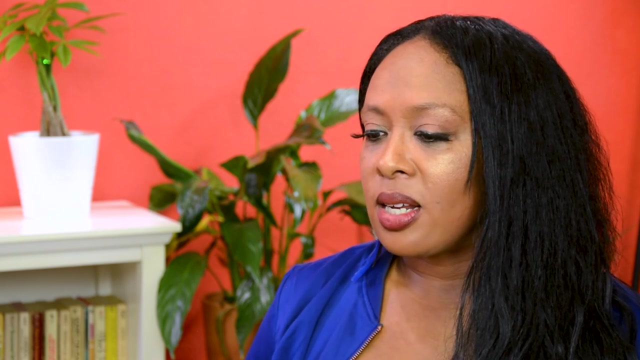 say, you know, um, shirley chisholm made, uh, um, obama, as well as hillary clinton, possible their their runs. you know so, um, and i remember in one of the interviews that she has, she says she goes. you know, essentially, that they may laugh. 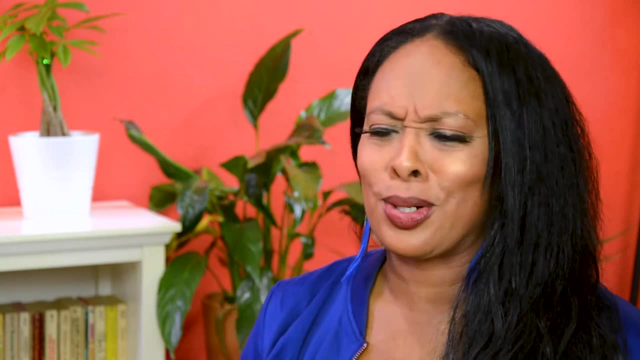 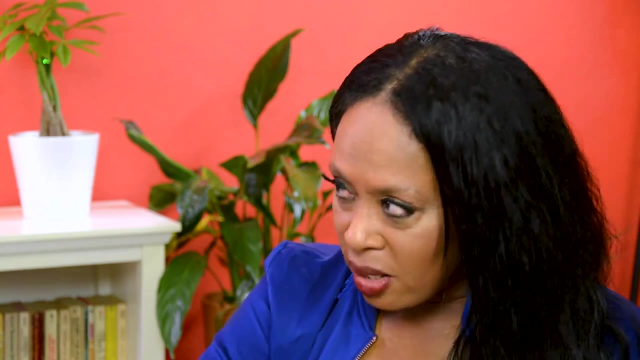 when they see me running- people like you know shirley white- she goes, oh you. they may laugh now, but they won't laugh the next time if there's a woman or a person of color running, because they can see that it can be done and it's so powerful that she stood there knowing that, with the 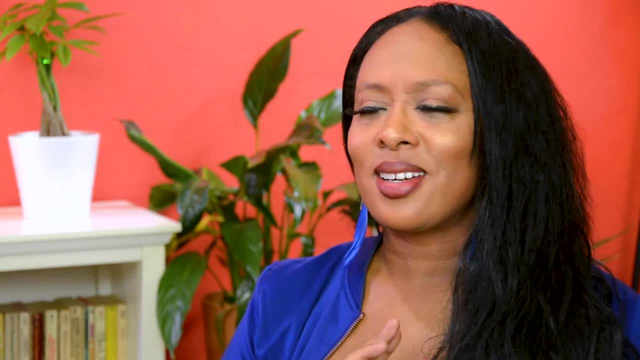 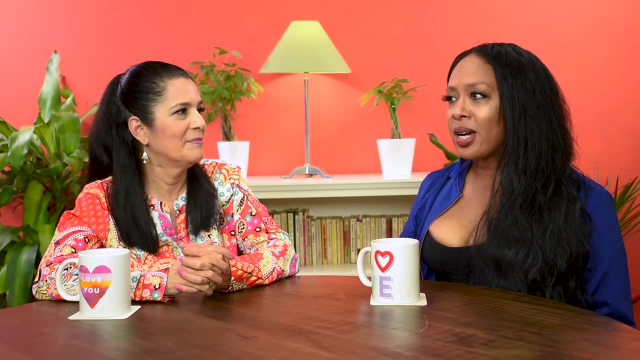 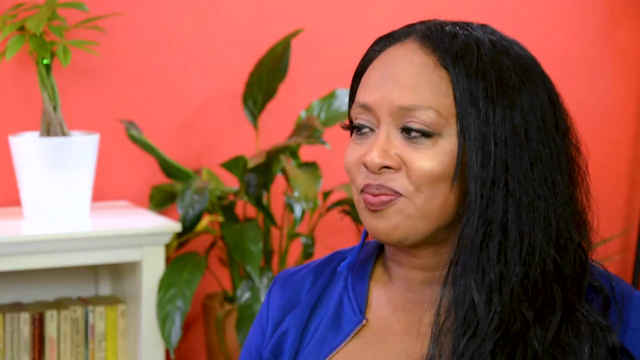 slings and arrows that were coming at her and she just stood her ground with a knowing, knowing my place in history, right here, right now. that, and you know, and so it's it- gives me chills. these women give me chills, y'all gave me emotion.